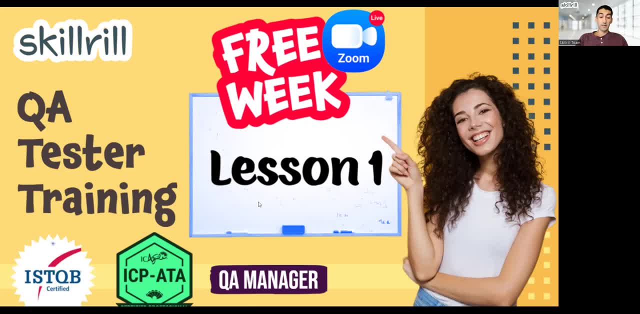 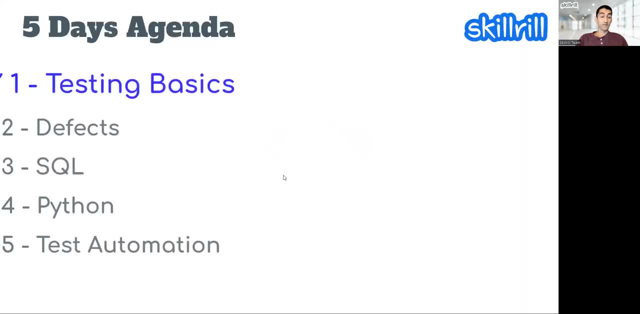 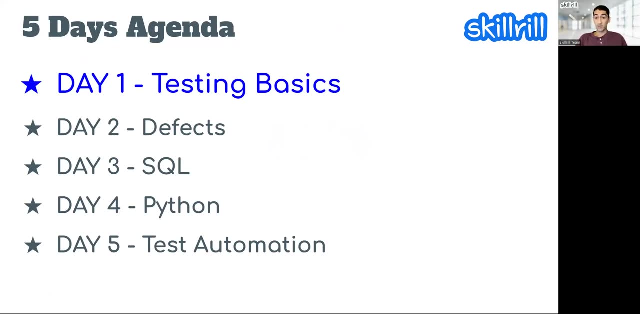 And today is one of those days, So that's about me. So let's just jump into the agenda of the five days, Right? So today we're going to focus on testing basics. So that would be. you know what is testing. 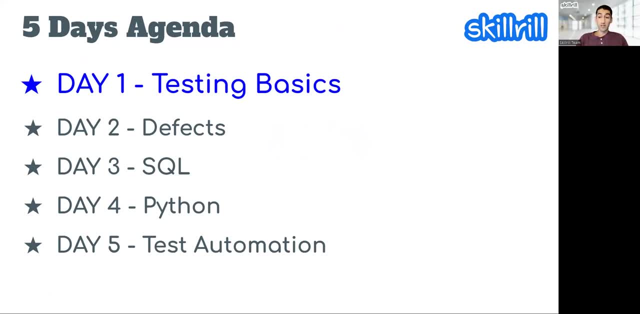 And what is software testing And also we're going to look into, you know, certain tools that are used in testing and the documentations that are used in testing, and so on. So tomorrow, day two will be dedicated for defects, Defects- they have their own lifecycle, and so on. 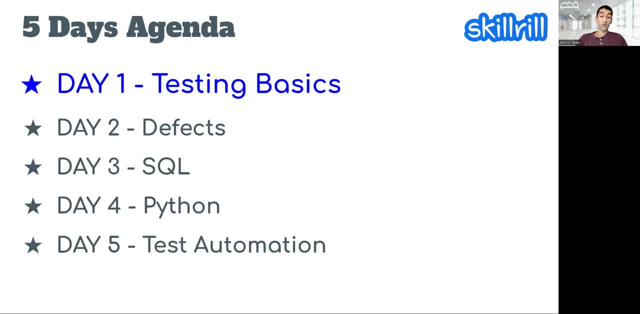 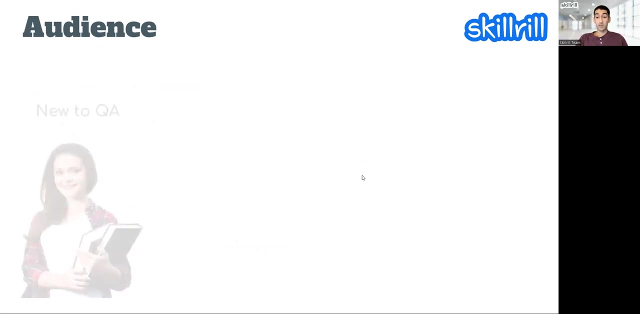 Day three, SQL. Then we'll do Python. You'll learn how to create your own scripts in Python, And day five will be Dedicated for a test automation. So let's just jump into the main content. audience today is very diverse, I have to tell you. 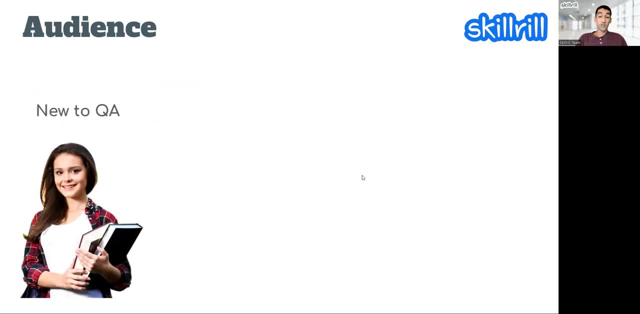 So majority of the attendees are new to QA, But we have also attendees who are already studying QA and attending boot camps or self studying, Some of them already in the market, actively looking for a job. and for those, good luck. And if those five days of lessons in any way will help you along the way in that journey, please share that story and we're going to be very happy to hear that. 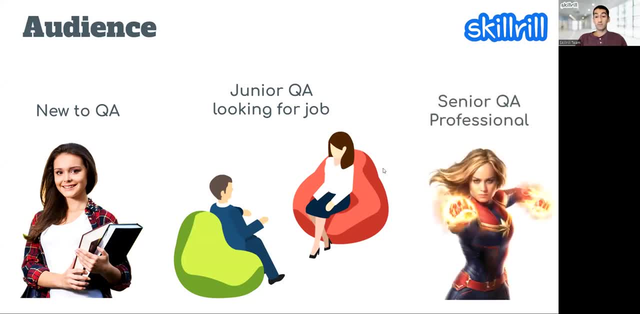 So we also have few professionals- senior QA professionals- in the audience And you know we welcome them. We welcome them as well. Everybody's welcome. We'll try to make the whole classes of each class as useful, as beneficial to every group as possible. 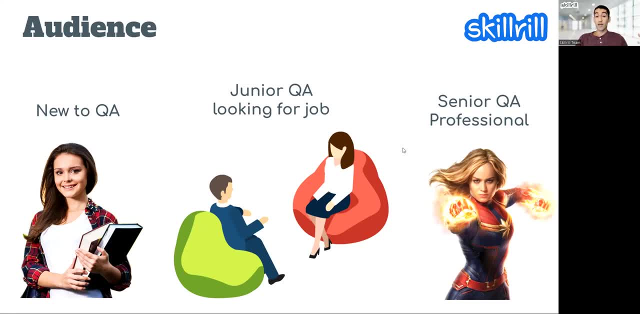 So questions, please put it in the chat box and I'll try to answer every each of them at the end. We'll try to keep it interactive as well, And I'll also share my contacts so that you can reach out to me if you guys have any questions or any feedback. 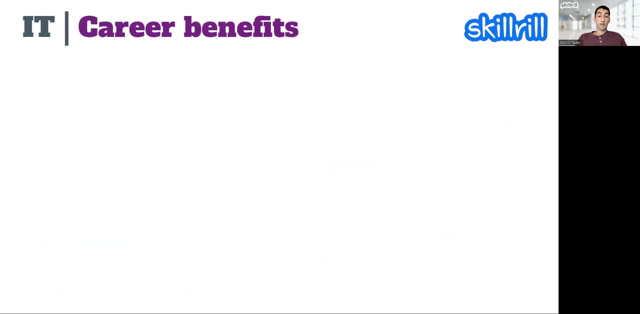 We'll be needed. So I want to start from the bigger picture here. So this particular slide is dedicated for those who are completely new to information technologies, who are trying to make their decision to change their career but they're not sure or they're looking for a motivation, basically, 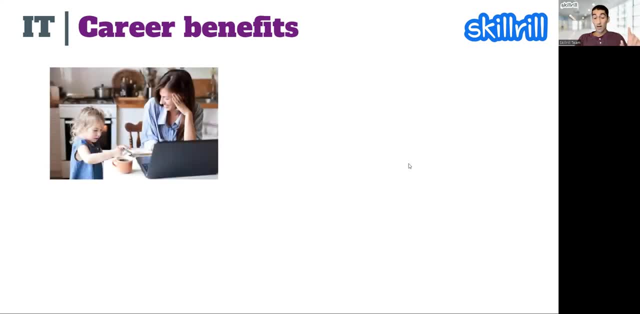 So I'll ask the audience this question. So imagine if you had a job offer today, two different job offers, With all the other parameters same, but one is working from home and the other one is working from the office. right, And I'm not guessing, but I know for sure that majority will be choosing working from home because this is the new normal, especially after a pandemic. you know, pandemic came harsh. 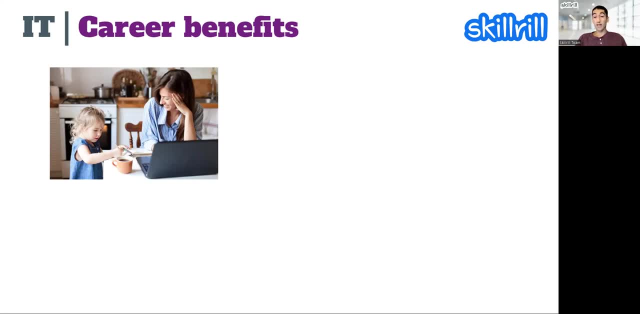 But it also taught the companies that people can actually work from home, especially the information technology Professionals. they can still do their job staying home and working from home, And if you're out there looking for a job, chances are that you're either going to get 100% remote job opportunity or hybrid couple of days home and couple of days in the office. great for work life balance. 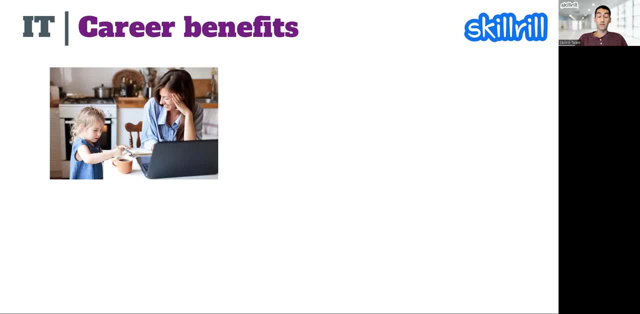 So so this is one of the short term sort of benefits that you can get right away if, if you will be In the market when you reach that point. So that's a great you know factor to take into account, Certainly. but apart from that, there's another. 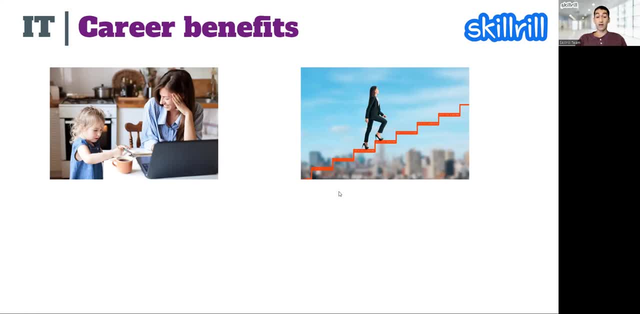 important factor that I get questions about. That is: is there an opportunity to grow? Can I actually grow, or am I going to be working as a tester, you know, for the next 10 years? So my answer is that there is tons of room for growth for anyone who is willing to, you know, work hard and work consistently towards their goals. 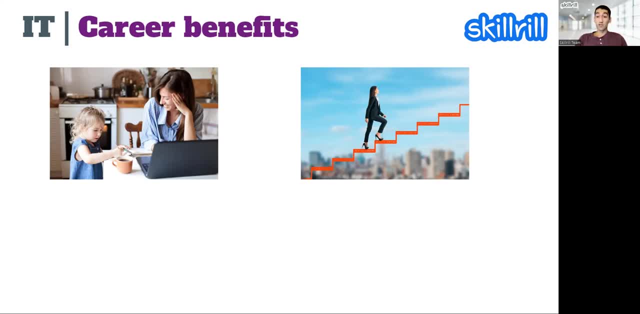 When I started working for US companies, I was surprised to see the- you know different positions, variety of different positions that you have at VP level, Vice President levels. You have, like, Assistant Vice President, you have Vice President, first vice president and senior vice president, executive vice president and all those, uh, you. 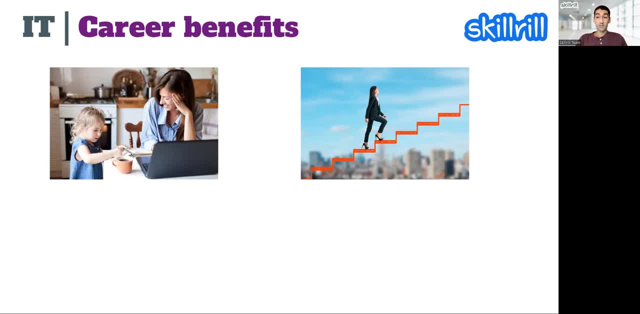 know variety uh of vp levels are are achievable, and and and of course you know that's something that you have to uh wish for and you have to work towards right. you have to put that goal and then you have to work hard uh towards that goal and that's achievable, i'm telling you. and 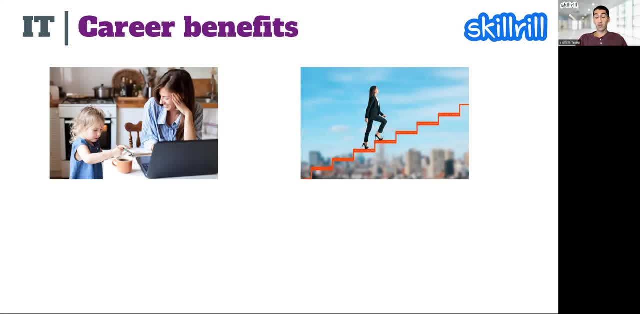 and then salaries, uh in at vp level that start from 150 000 a year and about in the united states. so, um, so i think those uh two factors are, uh, you know, one of the big uh factors that they're taken into account when making a decision to jump into the it career. 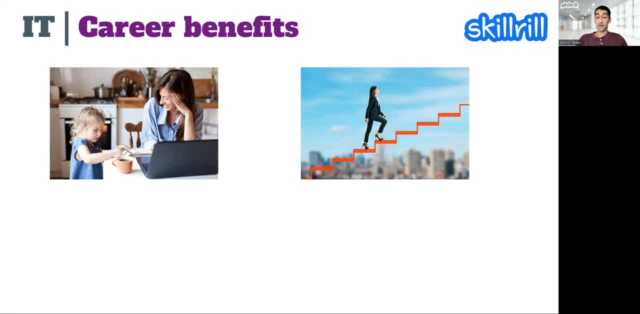 but apart from that, there are many other benefits uh that uh that you can also think of. for example, uh, paid vacations- right, who doesn't want to go on vacation? and then come back, and, and then, and then still get the same salary. so that's, that's a great uh thing that you can take. 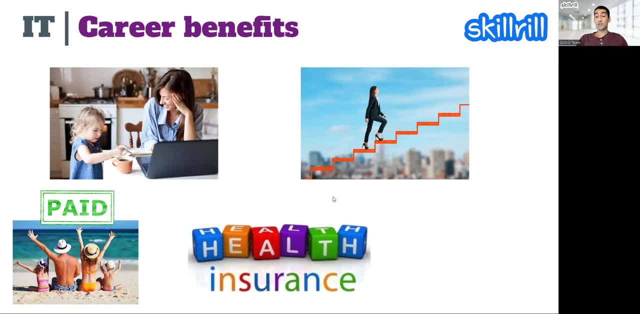 into account and also there's a health insurance benefits and also 401k that that will be on your retirement plan whenever you put a dollar and then the company puts: uh, you know another 50 or 30 cents additional to what you're uh keeping, uh or you know putting as a secure. 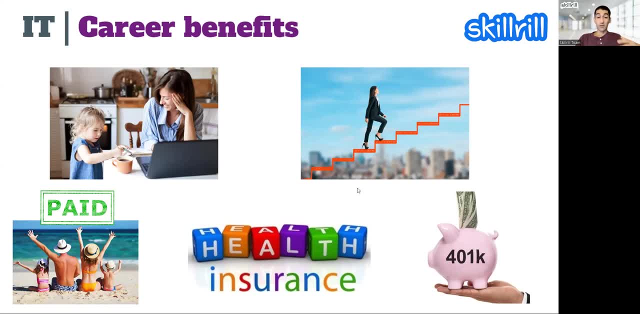 fund for your retirement. uh, that's something that i do. i mean, you know you can certainly consult that with your accountant, and uh, there is an arguable discussion about whether retirement plans are good or or bad, and maybe i'll talk about it in some other uh session, uh, some other day, but i personally 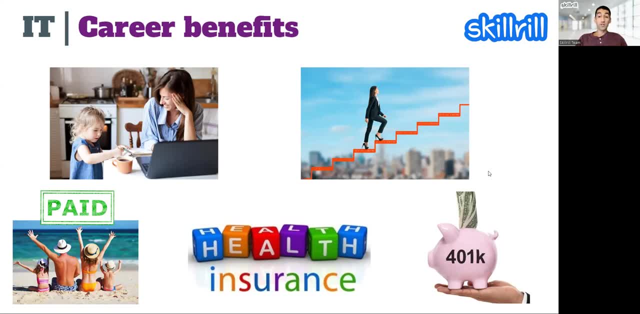 use that, sorry. so, uh, those are the benefits of the uh it- uh career, and i um, i think you know you should take that into account whenever you're in a position to do that. so i think that's a great way to do that. so i think that's a great way to do that. so i think that's a great way to do that. so. 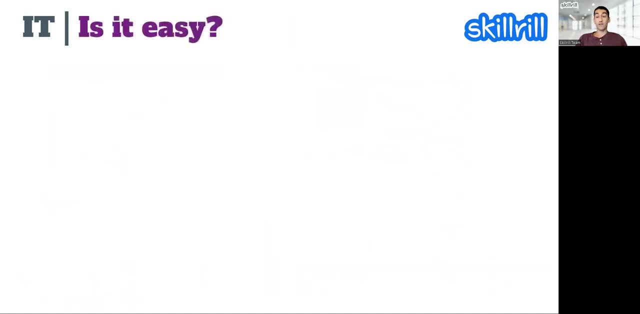 you're uh thinking or evaluating different factors, trying to make a decision. so let's answer the uh. try to answer the next important question here: um, that everybody has, and how difficult it is or how easy it is right now. i want every one of you just to think. 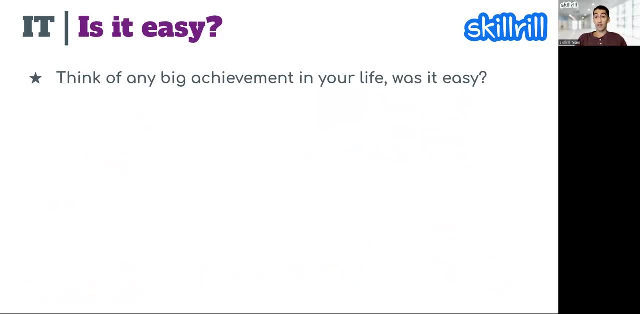 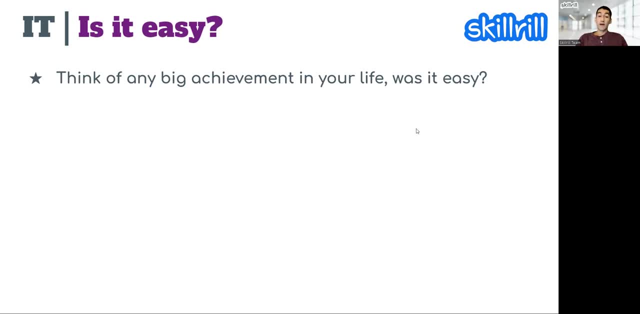 promotion and that's a good achievement. and, um, i'm sure it wasn't easy. i'm pretty sure it was not easy. you had to go through a certain uh steps. for example, you had to you know, put you know, have a vision or or a dream, and you had to follow your dream uh, and you had to set certain goals. 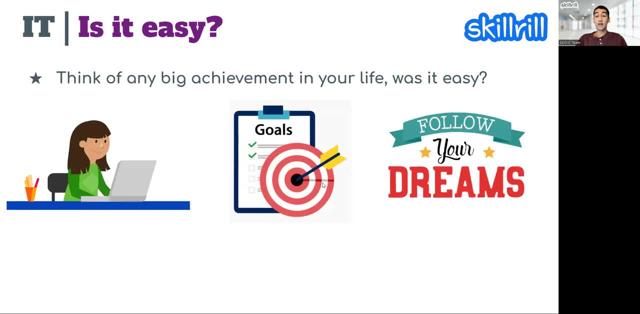 and um, you had to set certain goals, and you had to set certain goals, and you had to set certain goals and you had to work hard, right? so, um, well, guess what? the same approach, same recipe, would work here as well, because you were trying to change your career, you were trying to replace uh, other 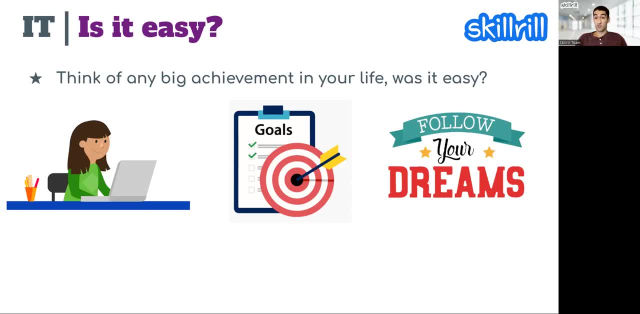 candidates who worked maybe for uh four years trying to get a bachelor's degree in it, uh, and then you were trying to compete with the with that uh other candidate, and certainly that requires that determination and um, and this approach that you actually used in the past to achieve other achievements in your life. so, um, 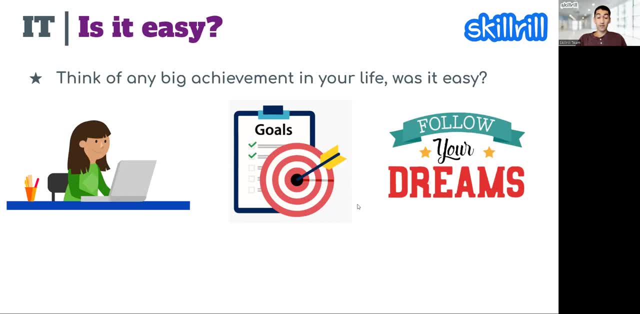 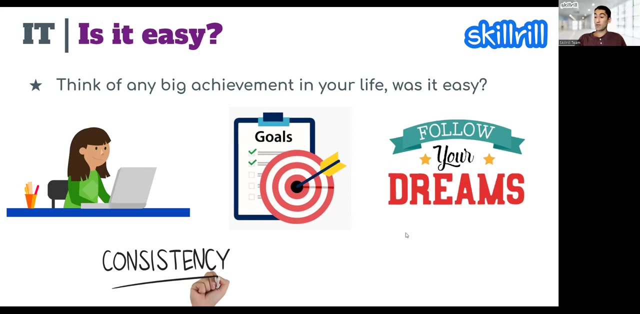 but there are uh two more important ingredients that i think that has to be mentioned here that makes this formula or the approach complete. that would be first. one would be um, um, uh, consistency. right, without consistency, you will uh not be able to uh complete. uh. or you know, you worked a couple of hours uh day one and then 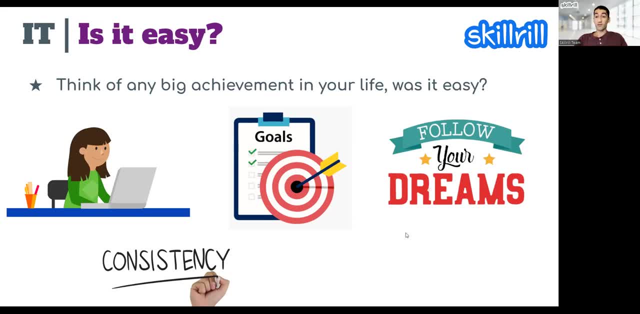 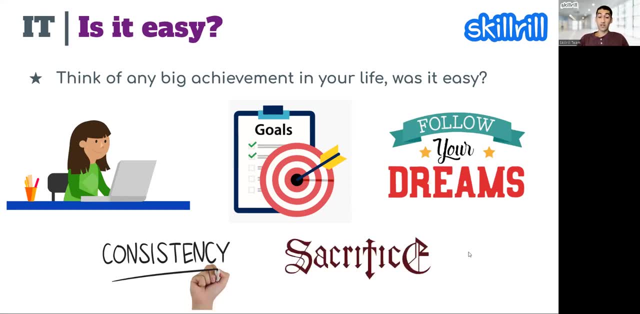 and then you skipped uh your lessons for the rest of the weekend. that's uh, certainly not consistency, and, um, and the other uh important factor here is sacrifice. so i'm certainly, uh, you know, not talking about any religious sacrifice or anything, but i'm talking about time management here, right? 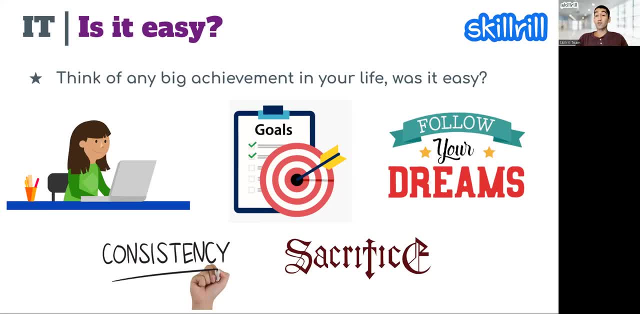 sacrifice. so, uh, i'm. so you have only 24 hours a day and, um, i'm sure you've been so busy and if you're trying to get into a new field, you need some extra time, um, to to study, and- and when i say sacrifice, i mean those little things that eat up your time. 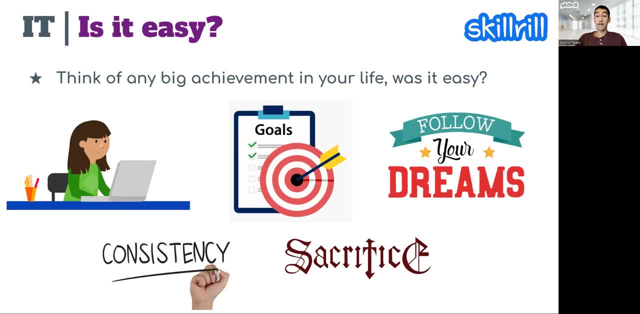 like maybe you should turn off or deactivate your subscription for netflix for a period of time, maybe stay off the social network for a period of time, like you know, stop watching those instagram reels and you know watching the random people doing weird stuff. so you're going to get back to the instagram or social network at some point it may, and then 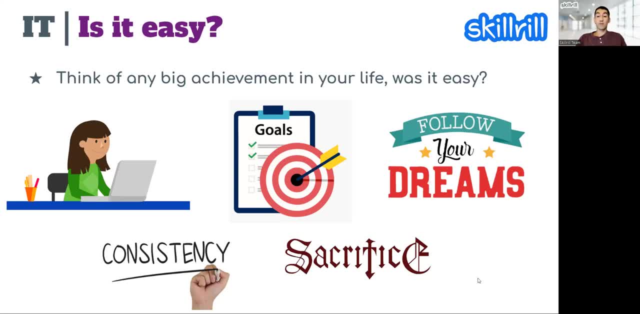 make that big announcement. hey, i started working for this big company, or doesn't have to be a big brand or anything so, but still, uh, you know any. you know, achieving any goal requires consistency, uh, and discipline, uh. so this is, you know, to make sure that we have 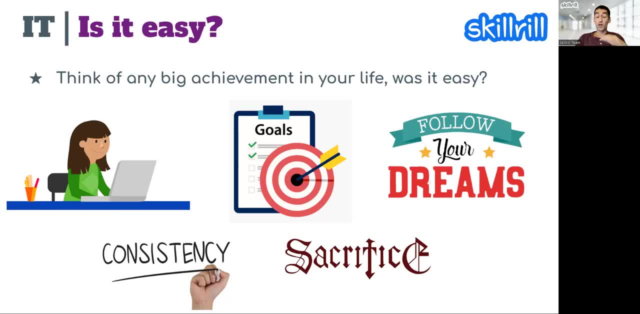 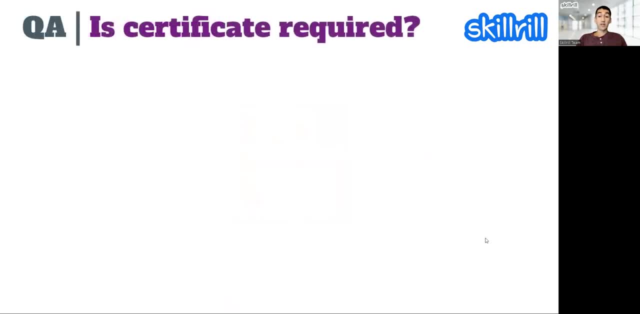 this correct expectations and correct mindset right from the beginning, right so? um. so it's, this is really important. uh. to mention now another frequently asked question that i get a lot- and i i saw that question also in uh, one of the facebook groups as well, um is is certification. 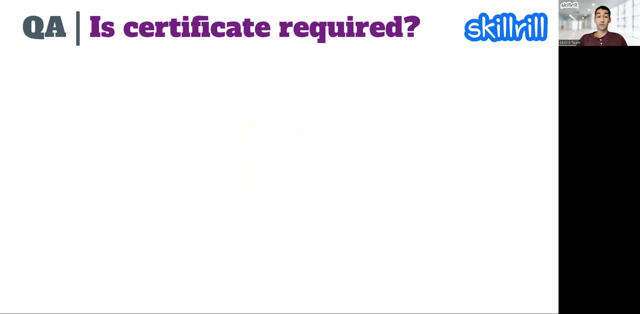 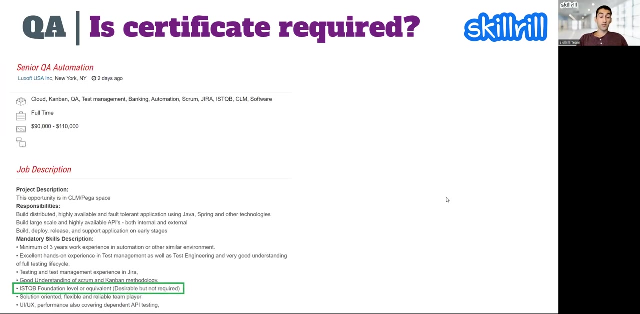 required, or is a license required. so if you were planning to become a doctor or uh, or um, or let's say, a lawyer, then yes, right. but if you're going to uh into into it field, no, you don't need to have a certificate, uh, but there's but right. so let's take a look into, uh, those two job positions. 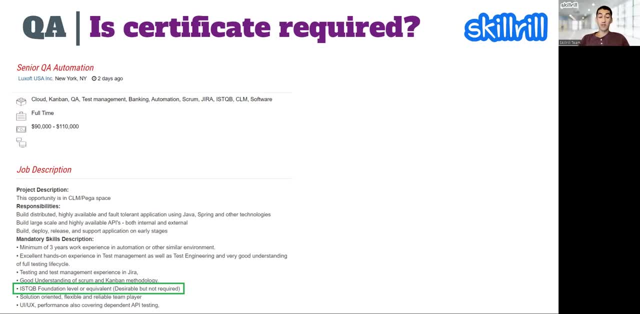 that i got recently. so this is a senior q automation position and i i caught this each and every one of these uh positions and i i captured this screenshot last week, i think- and and this uh position might still be hot, so those who are looking for, you know, job opportunities- you can still check that on dicecom. so if you look here, i highlighted 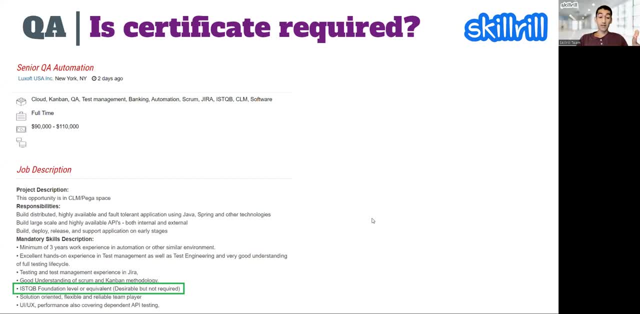 and it says isdqb- final foundation level- uh certification required, not required. desirable but not required. so so it's desirable. they're still listing that as part of their job opportunities and we're already in the second one, so we're gonna get back to the third position, so to be sure, and 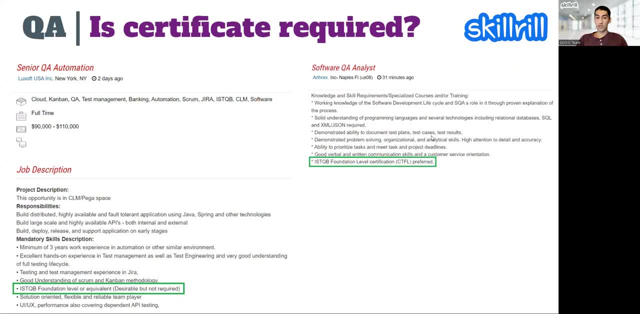 job description. here's another one that's more of a manual testing position and, as you can see, they also- you know, they're also listing that as as preferred, right? so the answer to this question is desirable, but certainly not required, right? so if you ask me, i say: if you're not in rush, if you're. 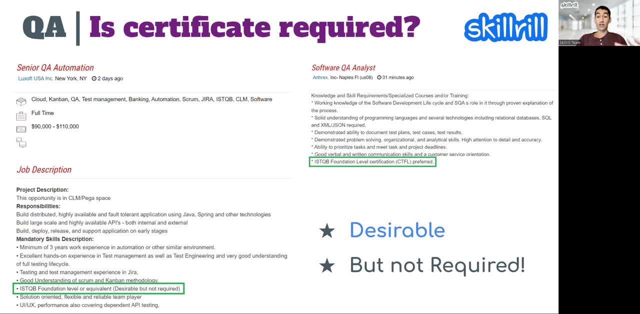 not, like you know, going to the market, and you need to get the job right now. if you're not in rush, then why not? you know, if you can do it. isdqb certifications or any other certification, but internationally recognized ones, though, right. so everybody provides certifications, but i'm you. 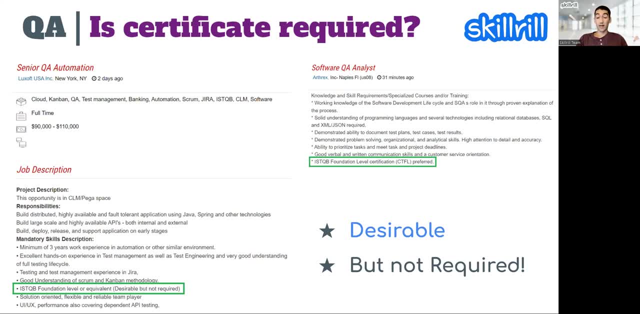 know, i'm really talking about the ones that are internationally recognized, like isdqb. so, uh, and they teach um a lot as well. i mean just to go through, just to get the job right. you know, if you're not in rush, then why not? you know, if you can do it, isdqb. 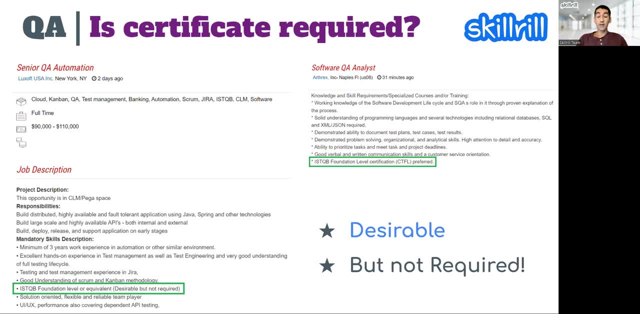 get the certificate, you have to study a lot, uh, independently. you can do that independently or get a coach and um, and when you get the certificate, you, you know when you pass that exam it's uh, i would say it's not easy as well. your level of knowledge in qa is is in a different level, basically. 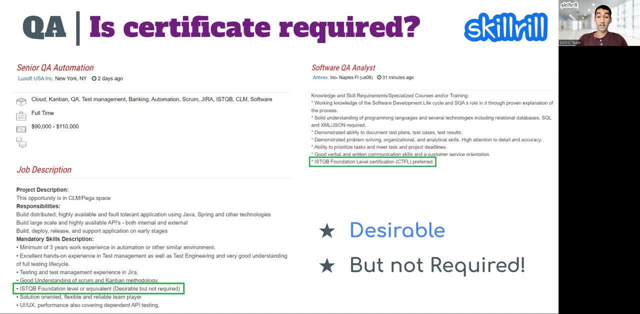 you're, you're gonna feel that some it may not be as practical as as a, as boot camps give you right like, like ours. so it's not as practical, but it's just gonna prepare you for the future or and also it's certainly gonna increase your chances of uh, of uh passing through those filters of like. 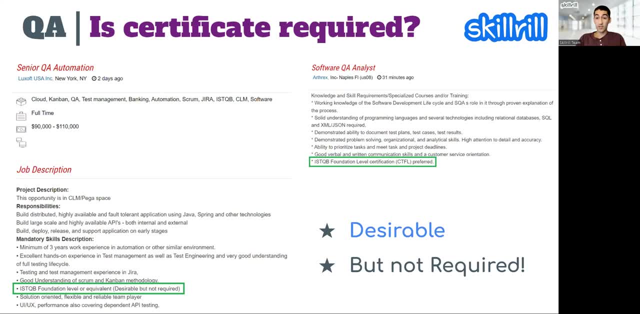 recruitment filters. so what happens to your resume is that you know it goes through those recruiters right and and it has to end up in the screen these days, not the desk right in the screen of of the qa manager or hiring manager- and they don't have the ability to do that right, so it's. 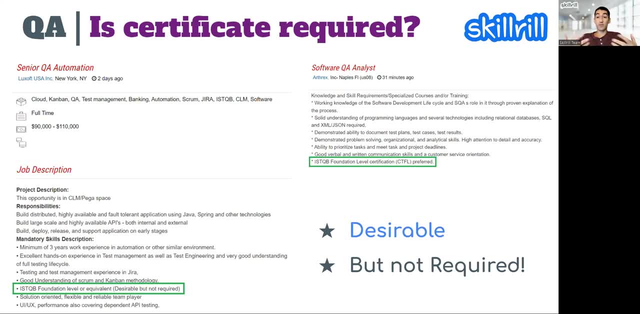 they don't have all day right, so they, you know they. for example, i myself, i get 10, 15 uh resumes and i i really have to select, i have to short list and there's no other way, because you know you can't be spending all your day interviewing people, because you know you have other tasks as 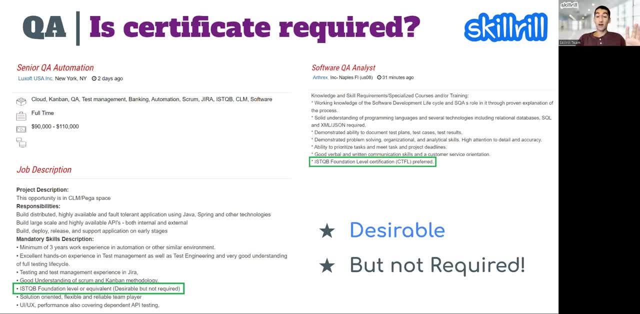 well, and you really hope, believe me, those managers, uh, and the- you know- recruiters really hope that those candidates end up being good, they, they end up being as good as described in their, uh, in their resumes, uh, so that you know they're also off the hook there. 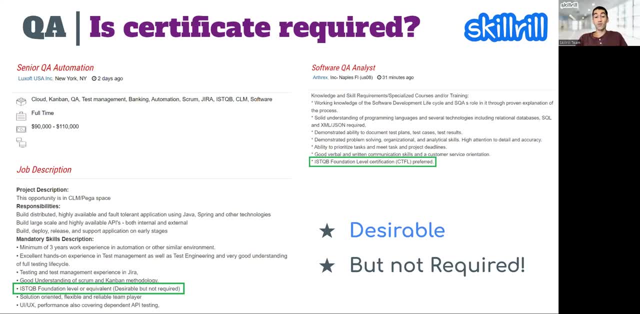 this job is done, okay, hiring process done. i mean hiring process so exhausting and and they really hope, uh, that they get the right candidate as soon as possible. so, again, desirable but not required. does it increase your chances of getting through those filters and getting you know? being short, 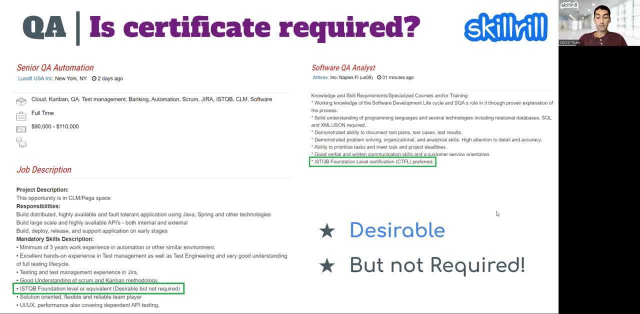 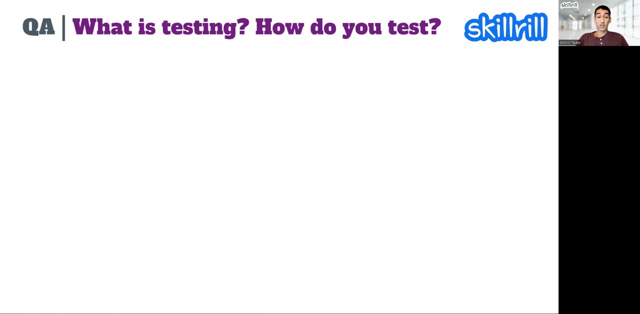 listed. yes and um, so, but certainly not required. all right. so now that we clarified some of the- uh, basic or frequently asked questions, we have the correct mindset, right, we know what to expect. we know that it's not easy and but you still have to work for it, right and um, we can answer the question of what is testing. right, we can jump. 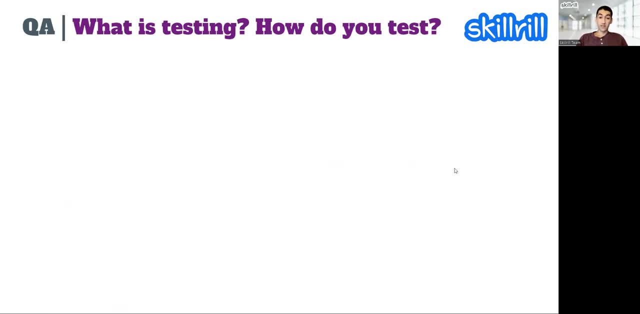 into the main topic of this whole uh lesson. so what is testing and how do you test if you can answer those two questions? you know, have the chance to answer those two questions and then the job is done. you're almost a tester, uh. so, um, what is testing? this is a very, very simplified 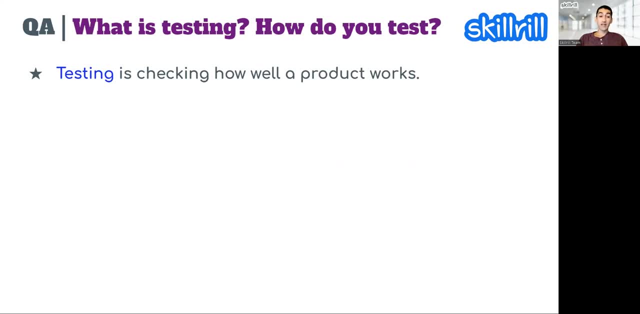 definition i'm putting here. testing is checking how well a product works, and i'm sure all of you have done this before. right, you have checked how well a product works and you know. you were in the supermarket, maybe in a walmart, buying some product and you were 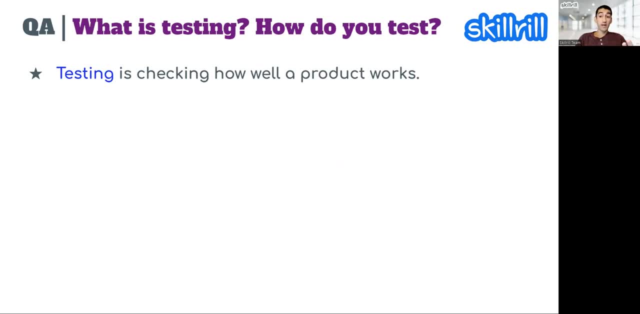 touching feeling and you know you were in the supermarket and you were in the supermarket- you're using it a little bit maybe- and what exactly was going through your mind, what kind of you know sequence of events or thoughts or algorithms were going, uh, through your mind at? 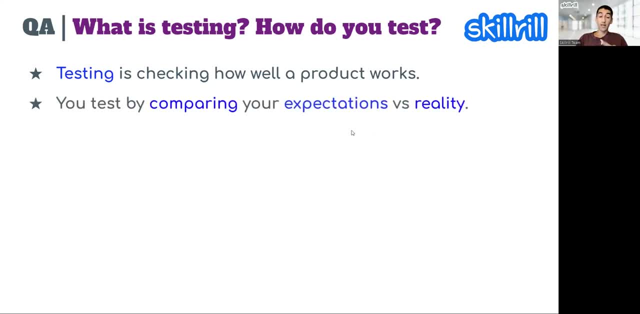 that point, you were comparing, right. what were you comparing? you were comparing your expectations versus the reality, and that's how you perform testing, right. this is what testing is about, and two important, very, uh, very important concepts that i want you to keep in mind: which is expectations versus reality, and there's 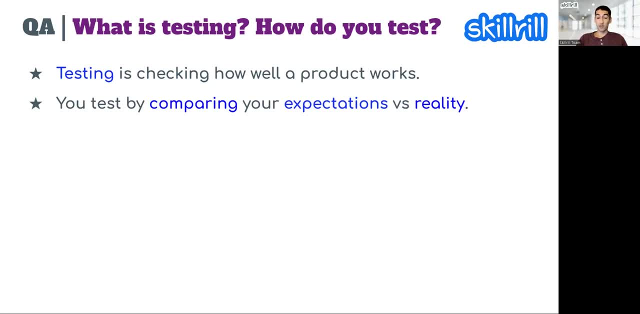 different way of saying it in actual software testing, but we'll get to that. uh, so now think of the um return period you get from amazon. why do you think is that? and what exactly you're doing during that return period? you're testing, right? you? you took that product, you're testing, and then 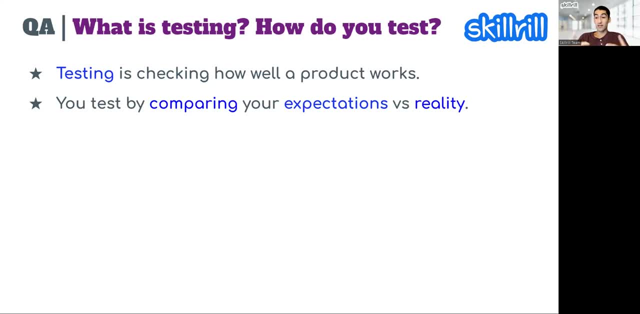 you're comparing your expectation and then with and against the reality. and if that, if that worked, if that matched and they were like, okay, this is, this is good, i'm keeping it. if it didn't match, then what you're doing is: you know you're gonna write this bad review and you're 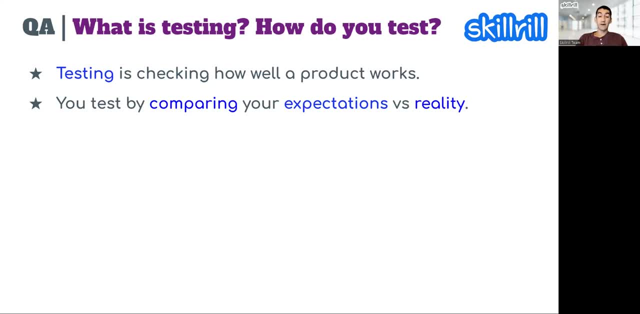 gonna return. right, give this three stars. um, so this is how you actually were performing the testing. now let's look into this fun, interesting example here in um in mid 1990s there was this- uh, you know- famous commercial about a mattress and a glass of wine, and this went viral and um the 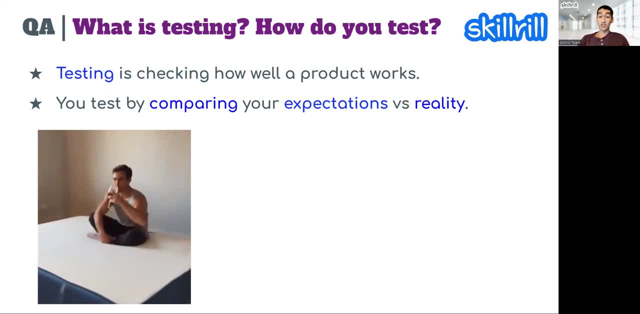 the, the product, the, the material that they were using is called tempera and it was originally created by nasa to protect the astronauts during space travel. and what is specific about this material is that it reduces the motion transfer right. the transfer of motion is reduced and this couple here- this is not the actual commercial, but this couple here is testing. 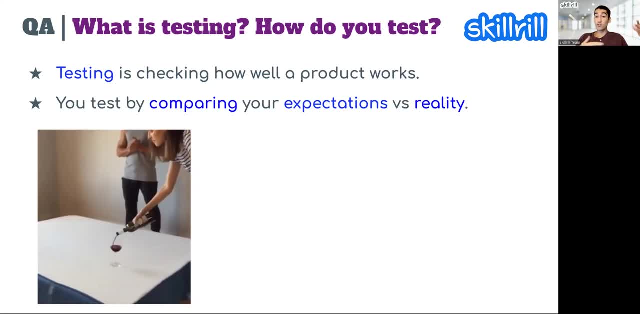 right, this is. this is what they're doing. they're they saw this commercial. commercial is their expectation. and they're doing similar actions. they're putting this wine, you know, the glass of wine, in the in one corner of the mattress and then they're jumping in the on the other. 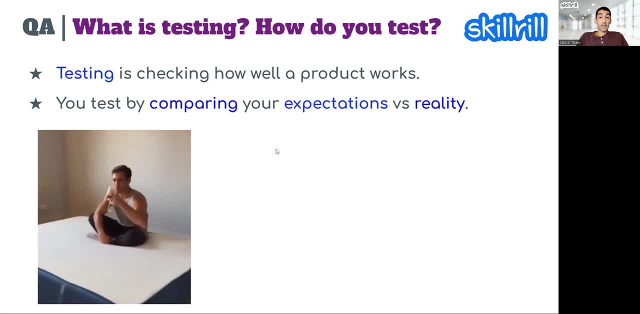 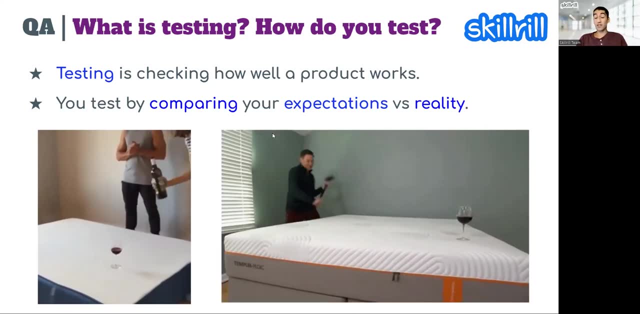 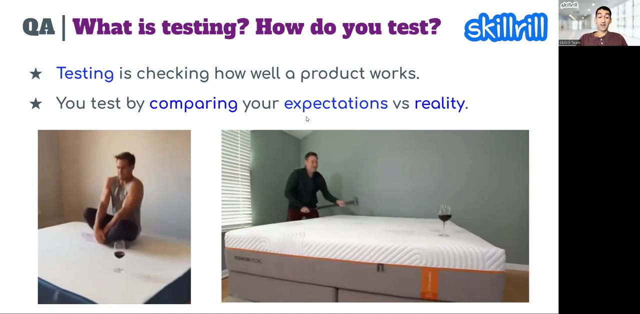 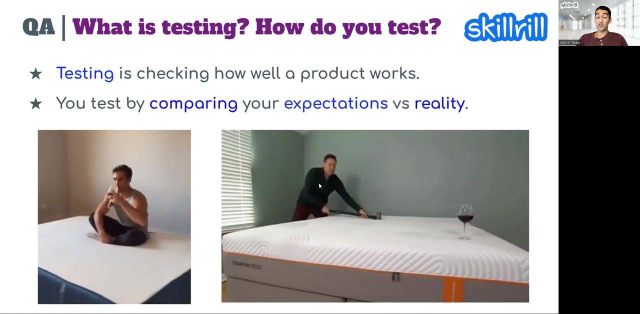 the other corner. so how else could you test that product? for example, this guy decided that he can, you know, hit it with a hammer, and several times so. so here's a question to the audience: um, how would you test? so imagine you're working for this company who makes the mattresses. 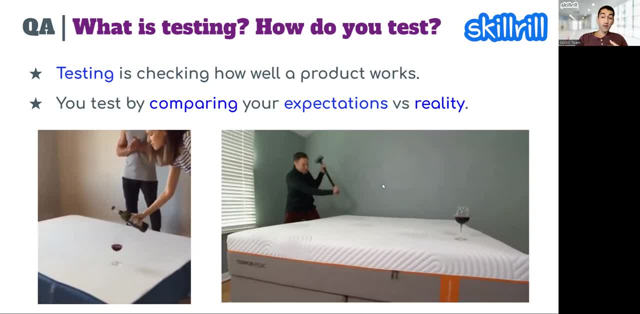 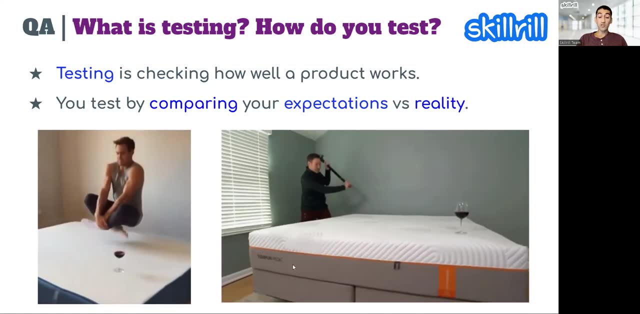 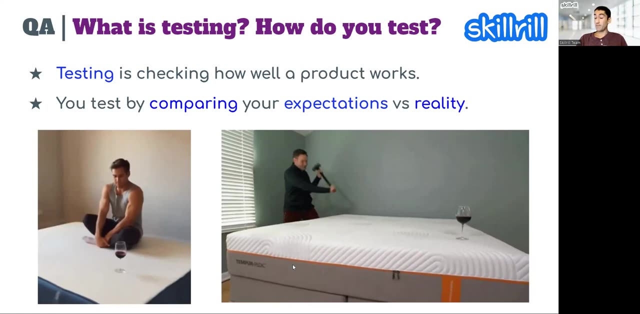 and how would you actually test? how you know if you can you come up with some other ways of actually testing the same scenario. so you can put your answers into the chat box and we call those different scenarios as test cases. so i'll give you guys some couple of minutes so this, so that you guys can type in. 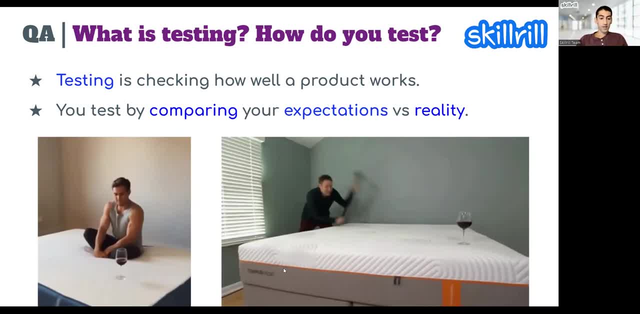 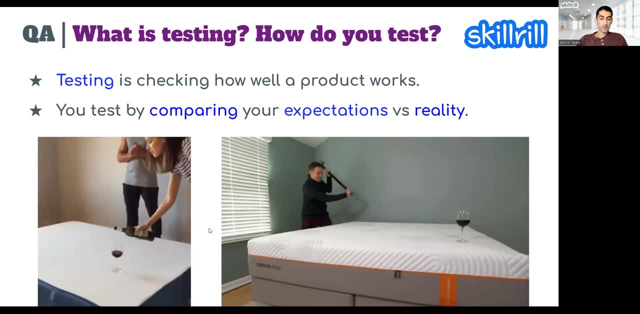 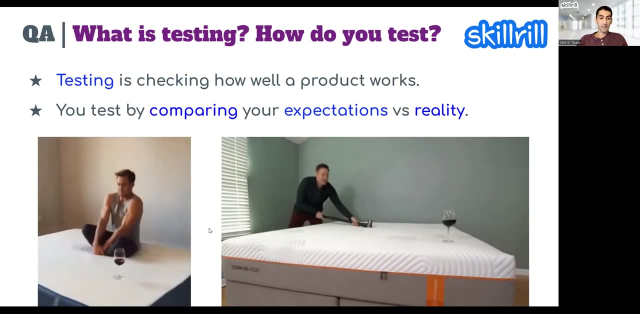 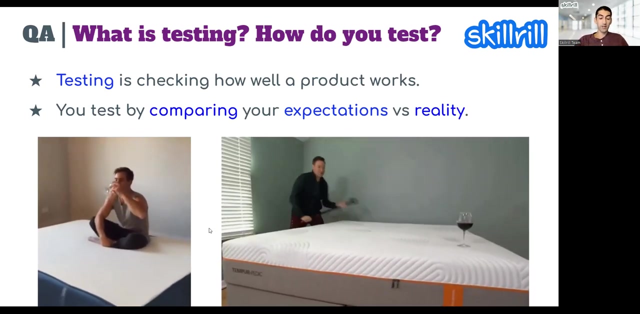 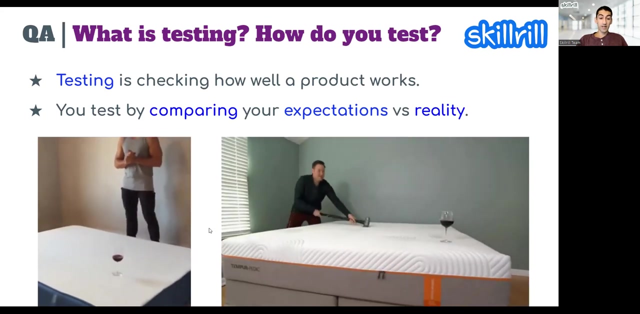 all right, all right. any any suggestions? all right, i see some answers here. use this for some times, right. use the product for some time. jump, great, okay, that's, that's great. yes, and you can also do exactly two people together. you can also do a backflip, that's right, you can. 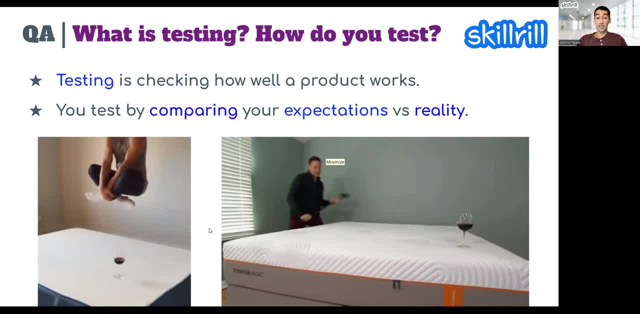 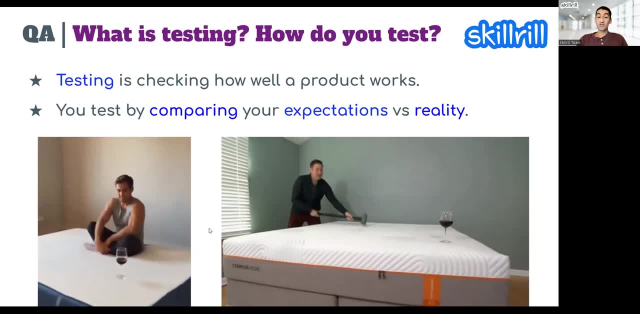 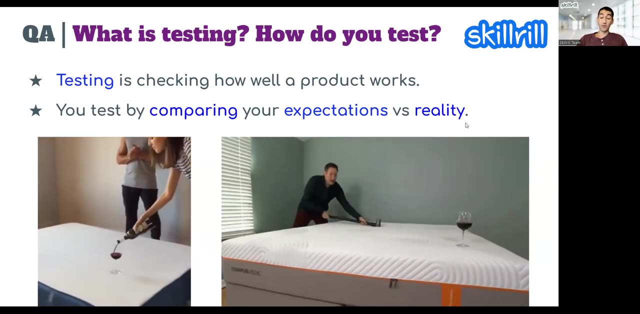 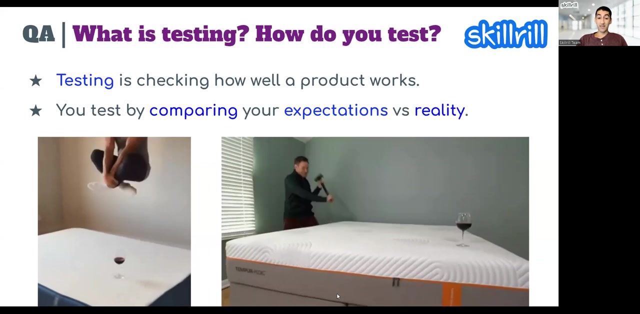 do a backflip and you can put a bunch of kids and then they can jump on it right, um, throw some stuff. yes, so, um, and uh, what else? yeah, you can use two glasses, uh, of wine. you can put one glass of wine on top of the other one and you can roll over. um, yeah, you can do all those stuffs and those are all. 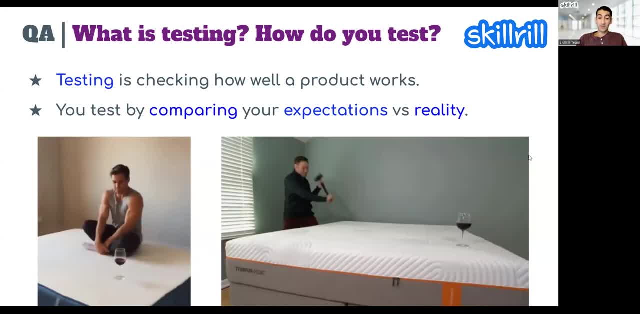 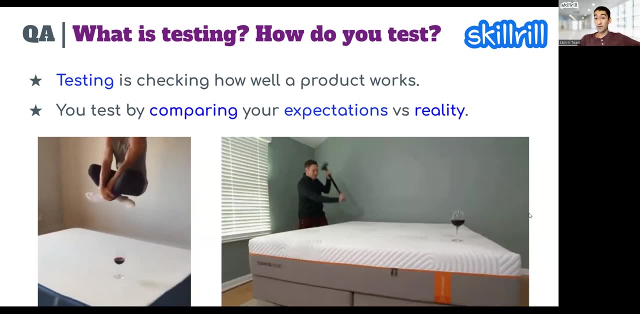 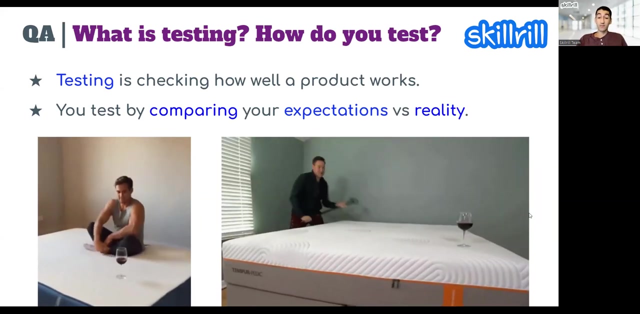 um, a different, different. put it there, yes it you see, uh. so what we call that in actual testing, uh terminology, is stress testing. now, uh, you know, do what you're doing for a period of time, or increase the pressure on the product to find that breaking point, right. i'm sure the testers uh off that company. they know the. 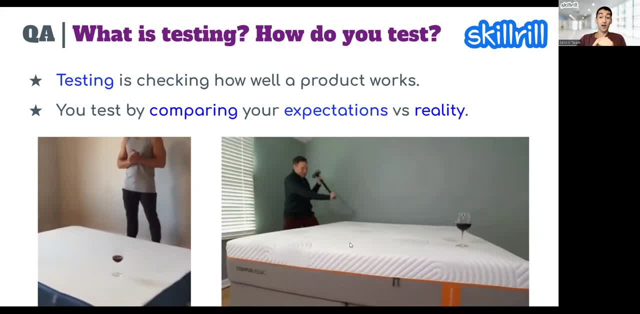 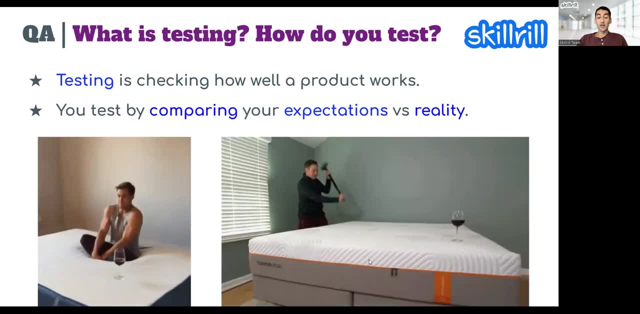 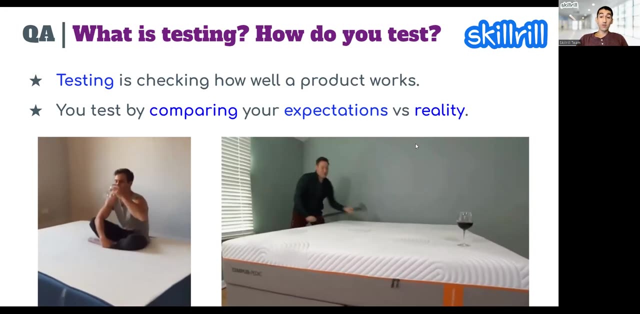 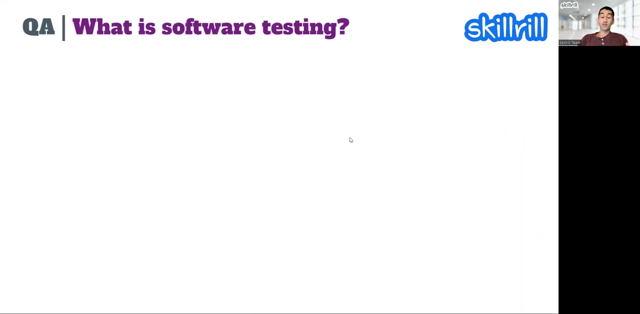 breaking point. know how close, if you jump too close, probably, to that, uh, to the glass of wine, it's going to spill. so you know, find that breaking point. so, um, so let's. so, now that we kind of clarified what, what is testing, so let's move on to software testing, right? so, um, you have been doing testing as, as a 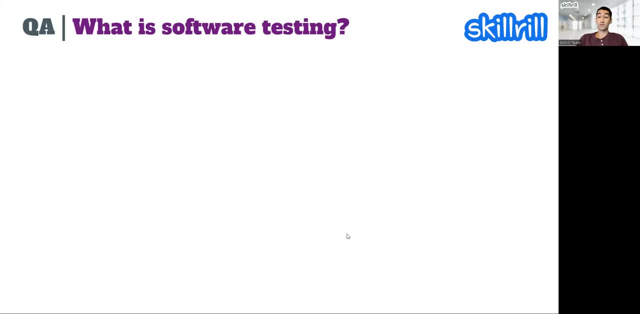 user all this time. but now you can actually do it professionally and get paid for that. so software testing, right? instead of the mattress, now we're thinking of the application, now we're thinking of the application. so here's the definition: software testing is verifying, right? those software testers use this cool word called verify instead of check. 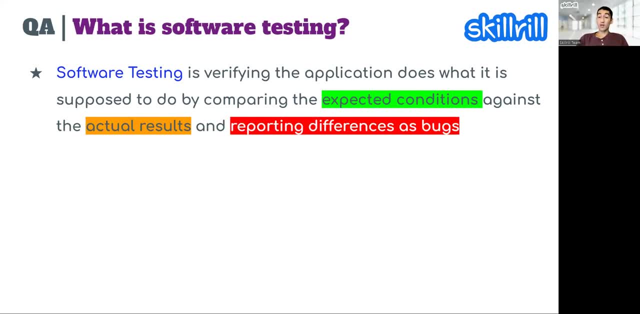 software testing is verifying the application does what it is supposed to do by comparing the expected conditions against the actual results and reporting the differences as bugs. right see, i just introduced you to a new concept. it's called bugs. so we're going to talk about bugs in detail tomorrow. so bugs, they have their own life cycle and bugs, they, they, they go back and 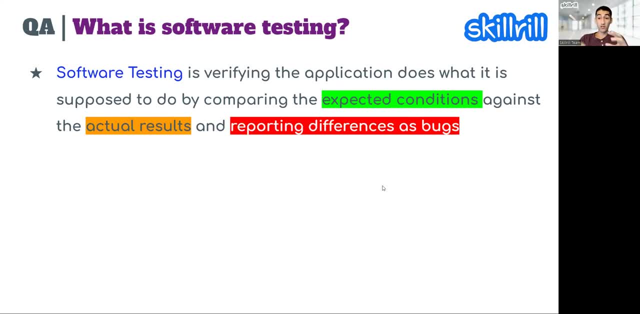 forth between developers- those engineers who actually type in the code to create the applications- and the testers. right, there's a special relationship between between the testers and developers. there's this hate and love. i'm just kidding, they don't hate us, they're just don't realize that they're in love with testers. so, um, expected conditions and actual results. 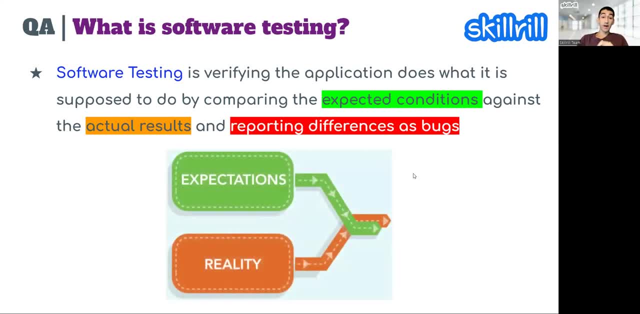 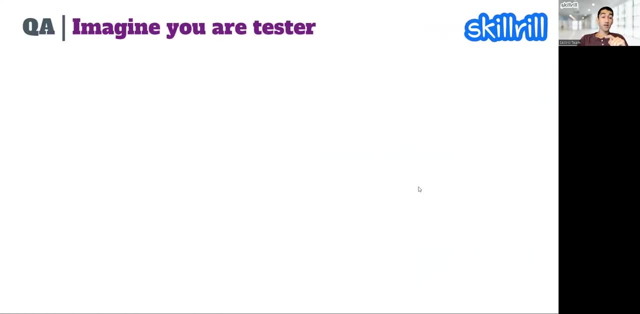 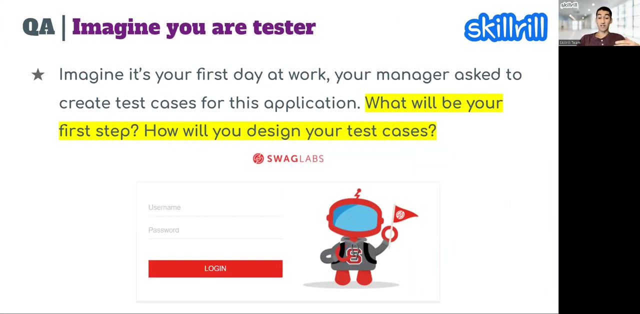 so those are the two important concepts that i want you to keep in mind because, uh, in the next slide, uh, i will try to trick you. imagine you're a tester and you got your first job. this is your first day. you're a little nervous and you know. you came up to your qa manager and asking like, okay, what's my task? what am i going to? 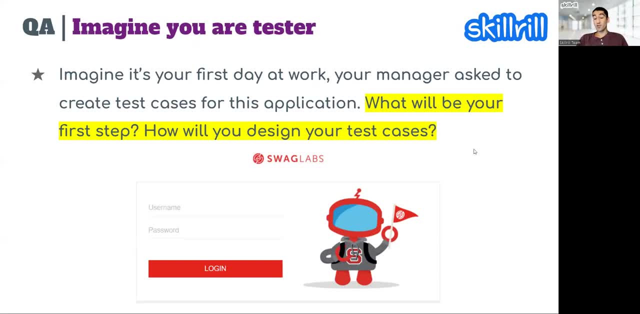 do. do you want me to do anything? right? so, and then your manager also doesn't know what to do. and then like busy and thinking like, okay, let me give you this test and i'm going to do this test. here's the application. just gave you this. you know? url of the application? uh, the address of the? 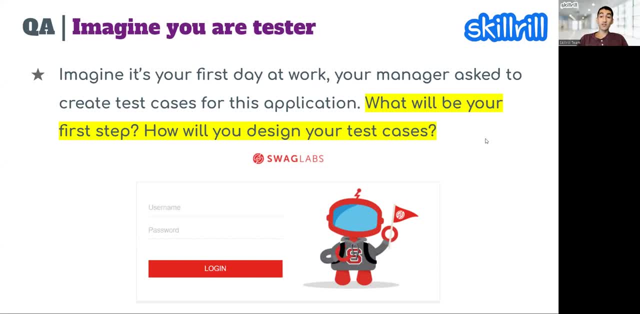 web-based application and saying like, okay, you will be assigned to this project. and then, uh, why don't you just think of how are you going to design your test cases? what is going to be, you know, your first step. basically, now, what will be your first step and how will you be designing? 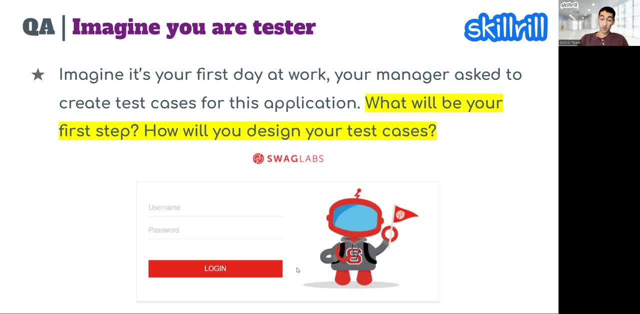 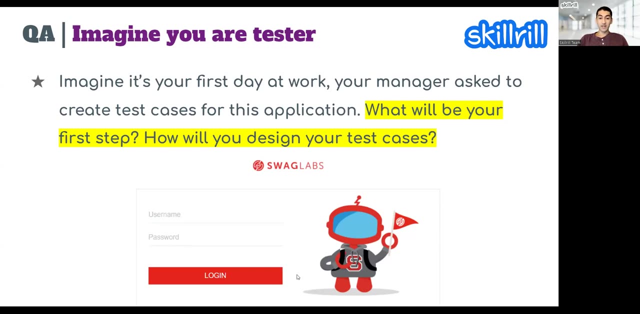 your test cases. so it's a question to you. so think about, think about that. what is your first step? how are you going to handle that situation? all right, all right, okay, i'm getting really really some really good answers. okay, exactly, that's right. yes, happy path: all right, so you're going to look for a happy path? 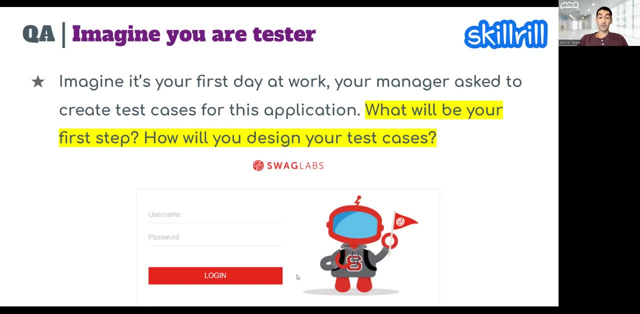 as well. all right, that's yes, you know that term. that's, that's great. read other test cases from other people. do that and great. so um, and this is also similar to some of the interview questions that you might get as well. so, uh, usually in the interviews as well, you're given a certain application, and not an application, but a scenario. 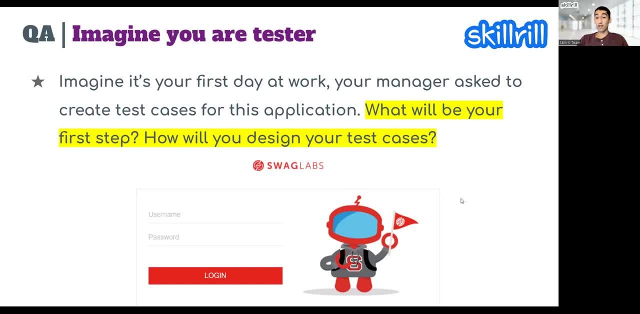 like you know, why don't you test a pen? why don't you test a broken calculator? why don't you test a calculator? or you know, broken toaster or whatever. um, common mistake that most of the you know new qa testers make is they jump straight into test case design and thinking of the scenarios that 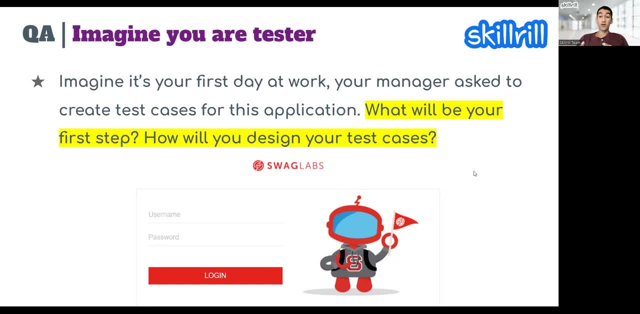 they could do, and so on, without asking questions, right? so good testers, they start from asking questions and your first step should be learning the product right. learn the product first. it's logical right? so if you know the product better, if you know the product better, exactly, yes, i can see some good answers. if you know the product better, then you can test better. 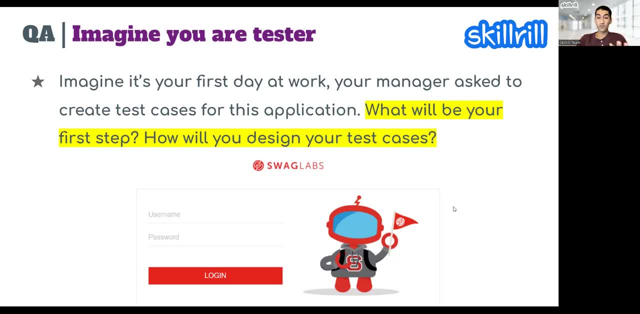 right, there are more chances that you're going to find those hidden defects. you're going to find those hidden defects. you're going to find those hidden defects, going to find out those problems and you're going to know what to test. actually, maybe this is an application that already exists and just small feature or part of this application change, so you. 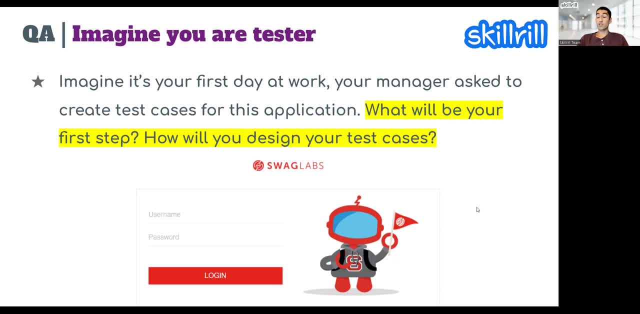 don't have to test the whole application, right. so you're going to have to understand the context, right. so your first step here would be to ask for documentation. thank you, yes, great answers from the audience. you ask for documentation if the documentation exists right and that shows that. 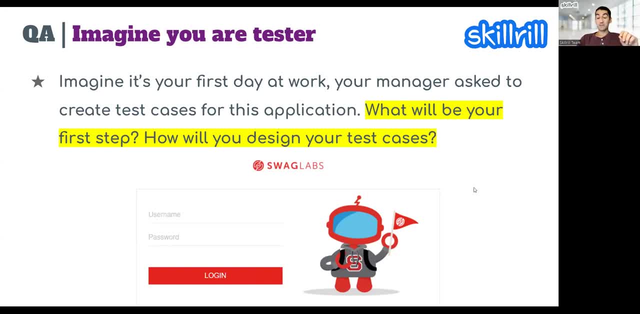 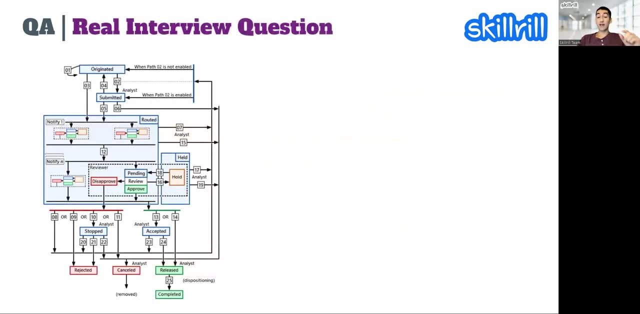 you know something, so let me actually give you another interesting question here. that's a real interesting question, and actually this is from my personal experience. this is one of the companies- one of the past companies- that I worked for, and at that point I was applying for a manual test. 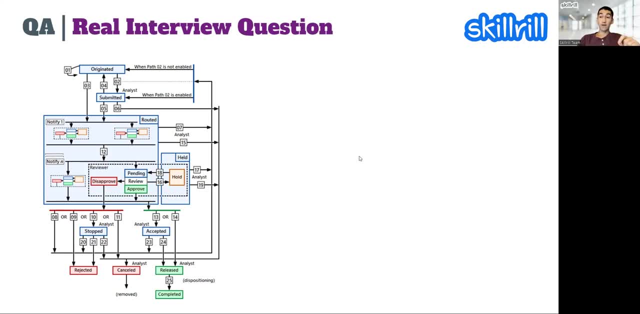 position and then I got my application and I asked for a manual test position and I got my. I got this question and the interviewer gave me a piece of paper. Those times it used to be more of a in-person and a panel interview with the other interviewers. 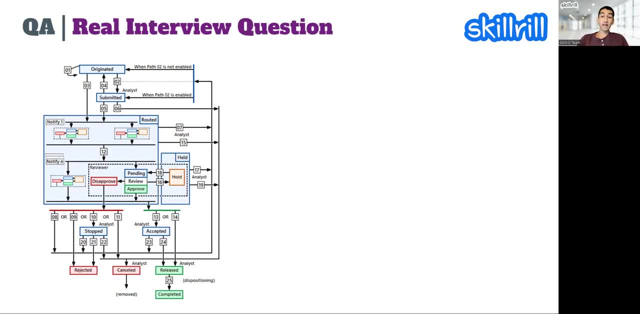 are in the room and then they're giving me the piece of paper with this diagram- not exact diagram, though pretty complex workflow, right? You see that there are a bunch of dependencies and then decision-making going on there, different statuses changing and then different roles- very complex. 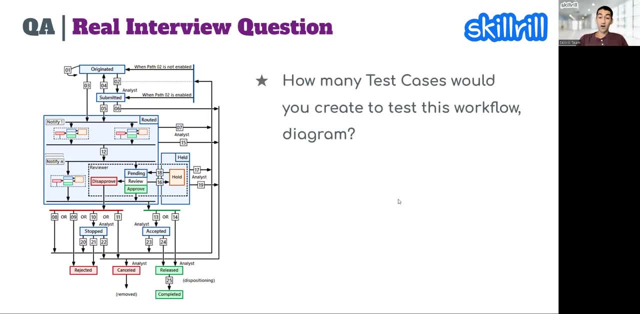 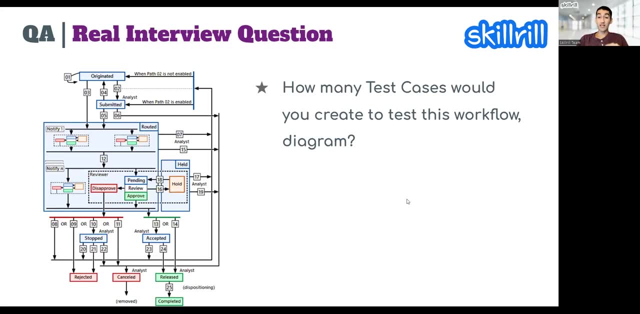 And look at the question that they're asking me. They're saying: how many test cases would you create to test this workflow or diagram? So, pay attention, They're asking: how many test cases would you create to test this workflow? right, I looked at. 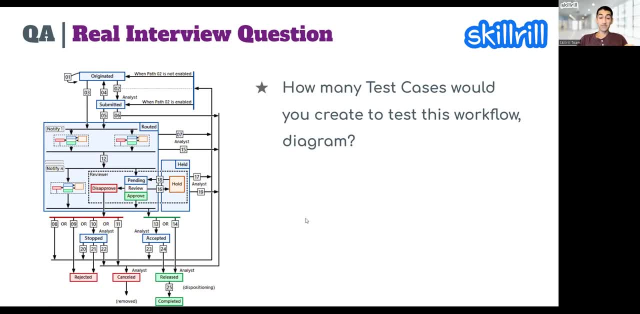 I looked at this diagram for a moment and then I quickly realized that they're certainly not expecting any number, right? So that's a tricky question, and they're not expecting you give any specific number here. That's just to check your knowledge of how you handle the testing process, how you actually 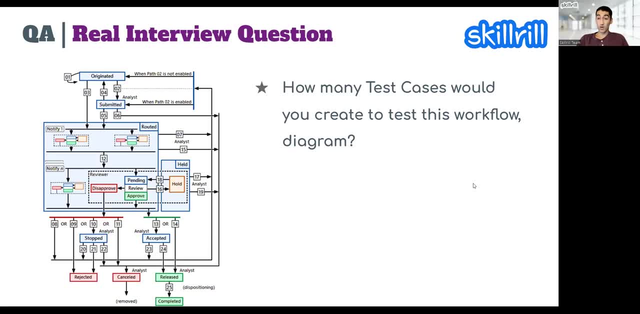 go through, what is your thinking process and how professional you are and so on. So here's how I answered. So I said thank you for the question And, as a tester, my reaction whenever I get a piece of paper with a picture or workflow- 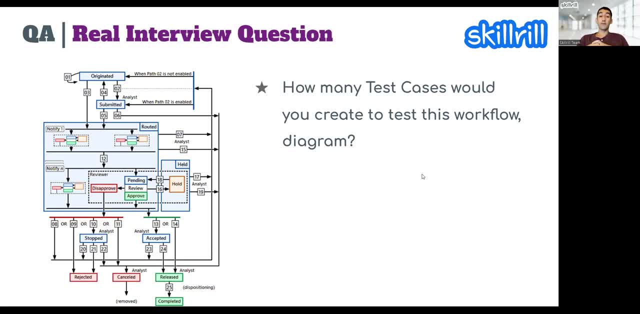 like this. my first reaction would be: is there more to it? Can you tell me more about this product? Is it, Is it a web-based application or is it a desktop-based application? Does this application has a graphical user interface, or maybe it is just the application? 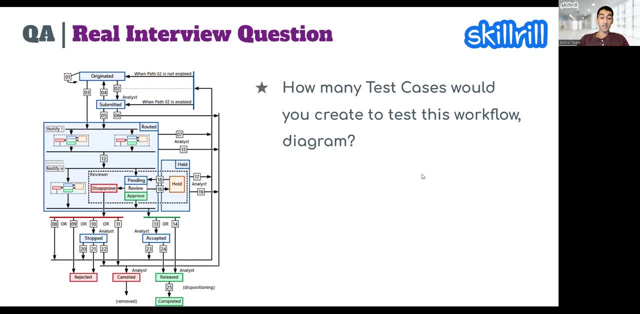 programming interface. Is there any other systems that it works with? it is integrated with? Is this a new application that is being created from scratch, or it's an existing application and some part of it is actually changing? Maybe there's like a before and after model. 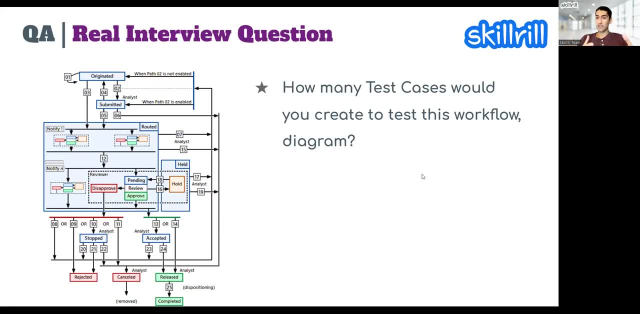 Here. Is this the latest version of this document or of this picture? Maybe it's outdated, whatever you're giving me. So there's so many missing parts, There's so many missing information before you can actually start designing your test keys, let alone the number of test cases. 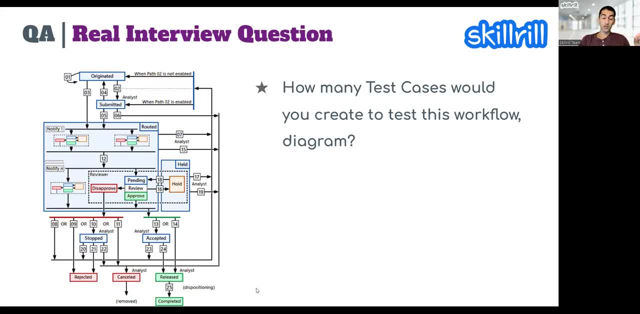 Number of test cases is the last thing that should concern any QA team. Okay, you can have a thousand test cases, 500 test cases, but if you're not testing all of the requirements, if your coverage is still below a hundred percent- I just introduced you to another. 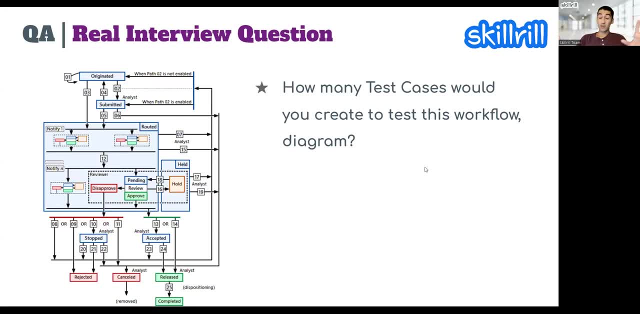 term here, coverage, right, Requirement coverage. So that means you know, are you actually testing all of the requirements that were in scope, right? Or maybe you're missing some of the requirements. So maybe you created duplicate test cases of 500 and they're just useless test cases. So the count 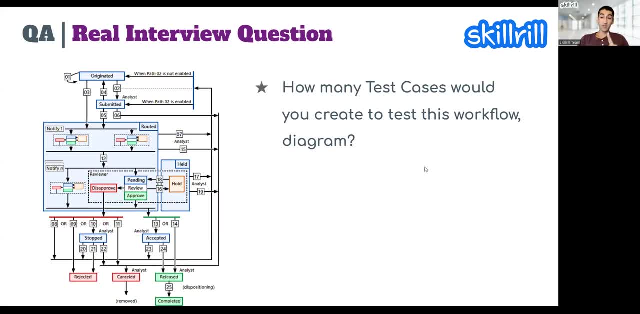 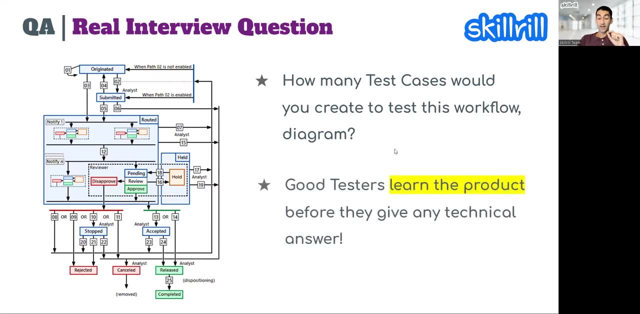 doesn't matter. What matters is the coverage right. But more importantly in this situation is your answer should actually communicate to the interviewer that the good testers learn the product before they give any technical answer. right, You have to learn the product, You have to ask questions. Good testers ask questions and good testers never trust. 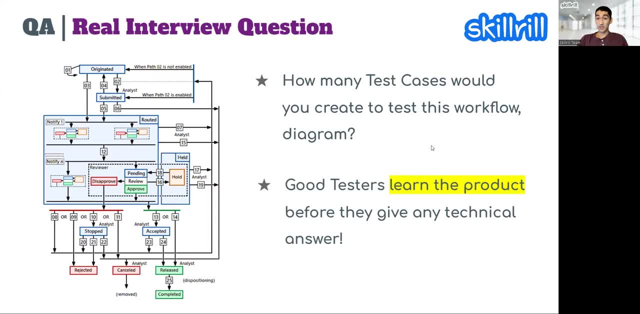 anything that's anybody saying. basically, you know, you have to verify, you have to verify, double check, you have to make sure everything's consistent, right, And then you do not assume Assumptions, also against your religion as a tester, right, If there is such religion. 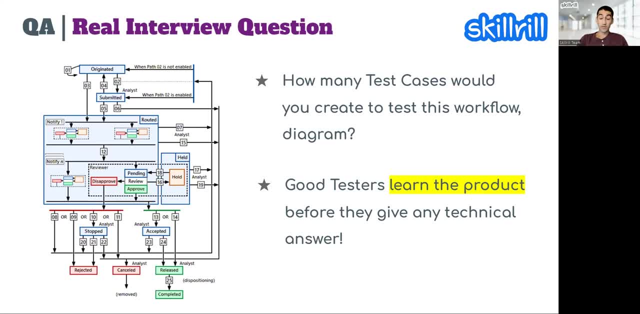 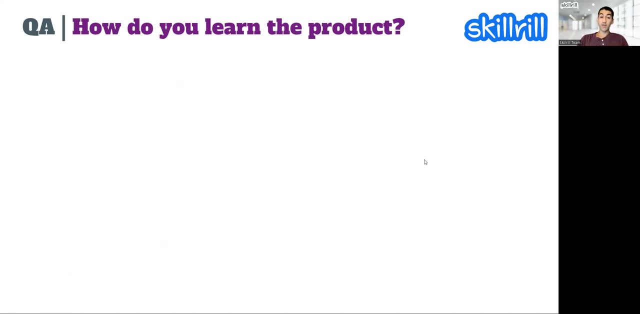 So you do not assume Testers do not assume, You're not allowed to assume. You have to work based on the facts, based on documentation. All right, so let's now jump into the next step. I think a follow up question here from the audience who are new to QA World is OK. 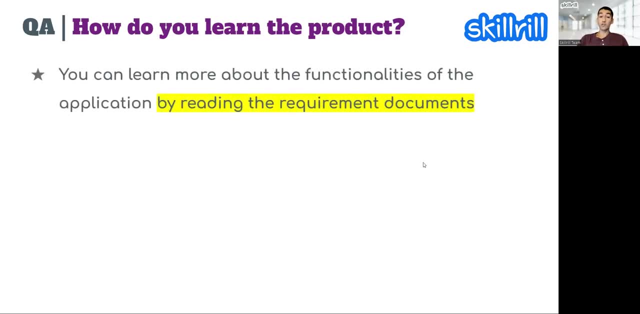 How do I learn the product right? How do I learn the product? So you'll learn the product. You'll learn about the functionalities of the application by reading. surprisingly right, By reading. So you read the book, you read the requirement. 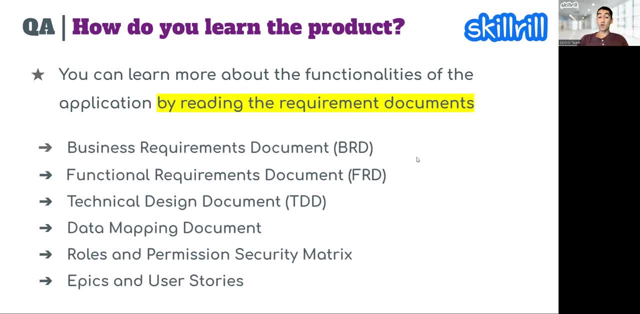 document And there are many different types of requirement documents that you know you might be given on your first day or during your QA career. You know it's the start from business requirement document And some of them might be actual documents, Some of them. 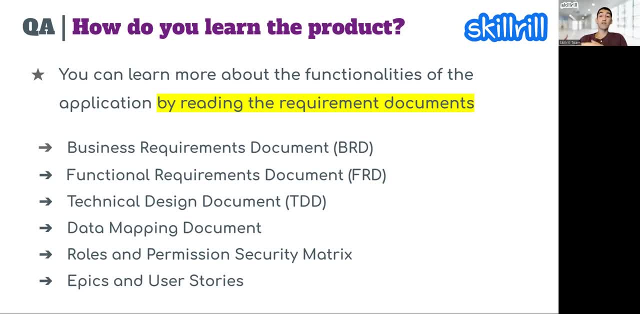 might be just information that's electronically saved in the in tools and certain tools, test management tools like JIRA, for example, like in the form of user stories and so on. Right, Certainly don't want to complicate this at the moment, But the purpose of those documents is. 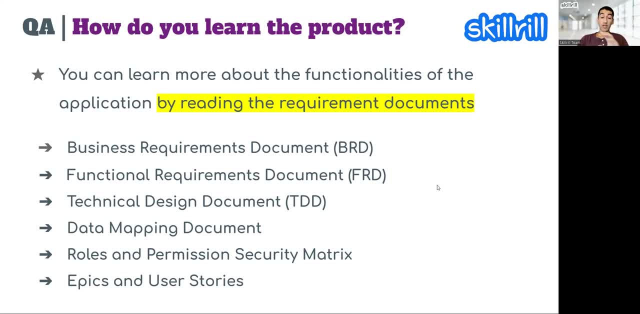 To describe how the application works, to describe specific features, functionalities of the application under test right, the application that you're planning the test, and then when you read those documents now you start understanding the application, you get better and then sometimes you reach the point that you're actually going to understand the 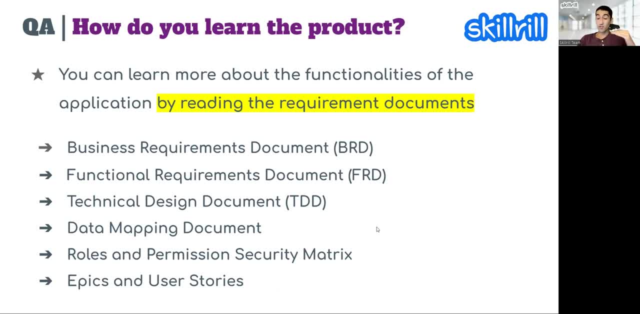 application better than the developers, better than maybe even the users, you know, because the information changed. right, users requested something and then it was converted into some, uh, some documentation by, you know superman, a guy called business analyst, and that business analyst interpreted in the way they, uh, they think, and then information changed along the way and 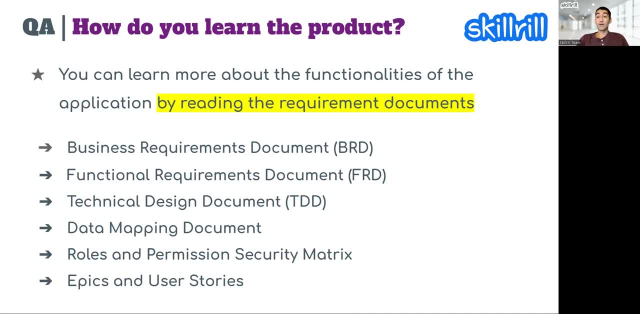 then. but this is the you know application that's created and users eventually accept right to certain extent, um, and then you at the end of testing actually become a subject matter expert in testing, and then you and then those users actually reach out to you, and then they involve you in the meetings and 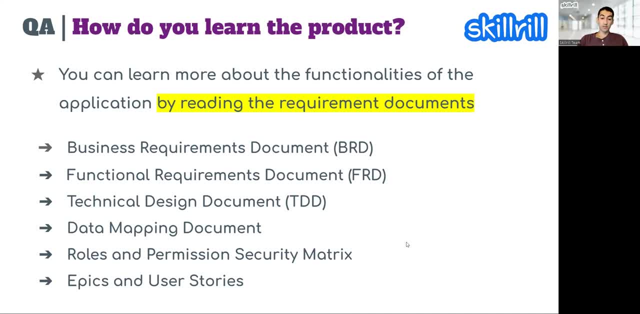 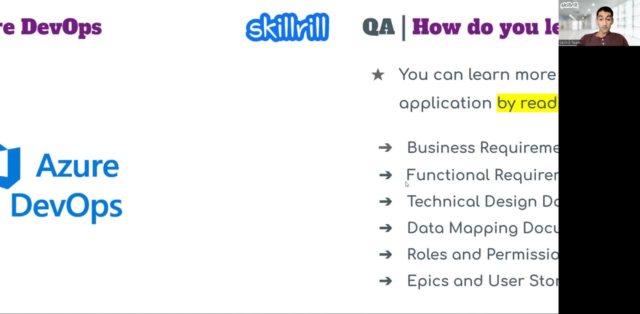 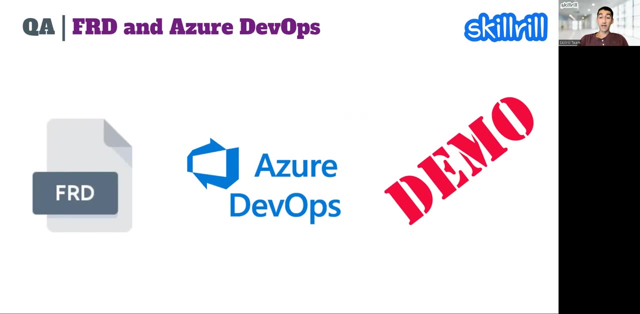 ask you to help out understanding the application better, so that they can test as well before they start using, before they accept. so now let's assume that you ask the right question from your qa manager, qa lead, and then they provided you this documentation- functional requirement documentation- and that's what we're going to look at in the next few minutes. 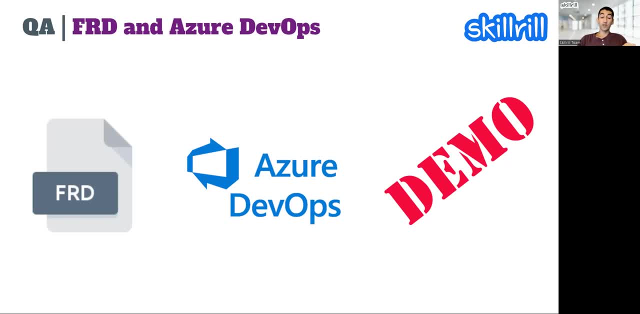 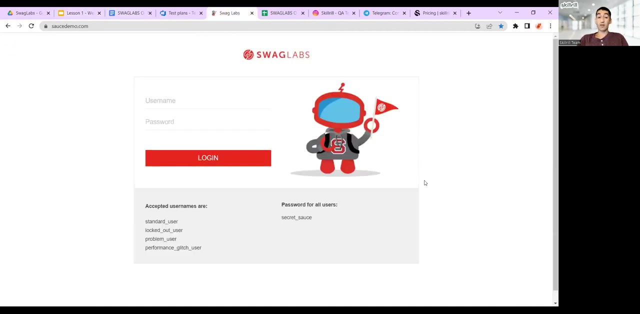 um, again in terms of you know the process for accessing the document. if you want to servivence that application via with pdf, you can take away just using this. not sorry, this security Region耶. nah, it's an application that father could accomplish when your CA manager sent you the document. 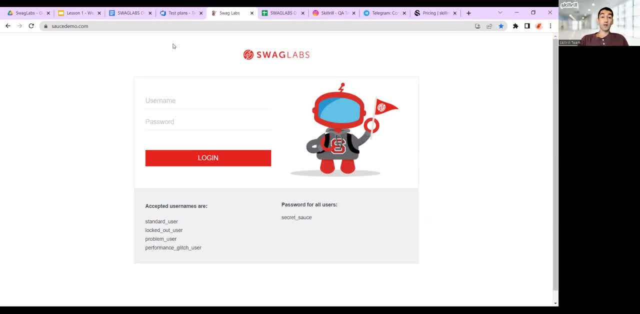 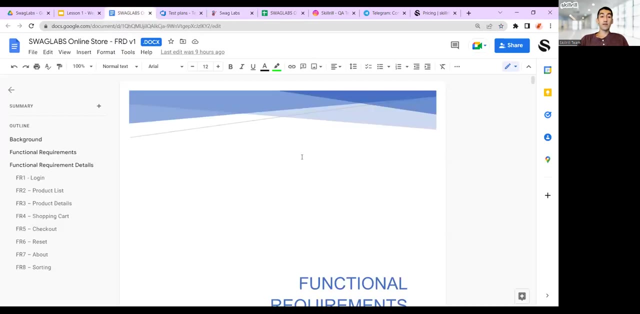 you can see everything right, so right now. So, test environment: that means that it's an application that you can test without impacting the actual users, right? So here's the typical functional requirement document. Here's a typical functional requirement document. So, again, the purpose of this document is to explain you how the product works, right? 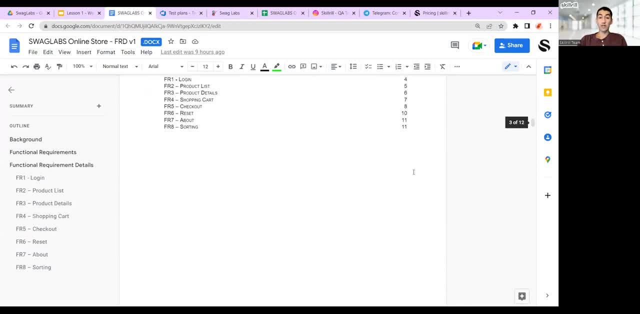 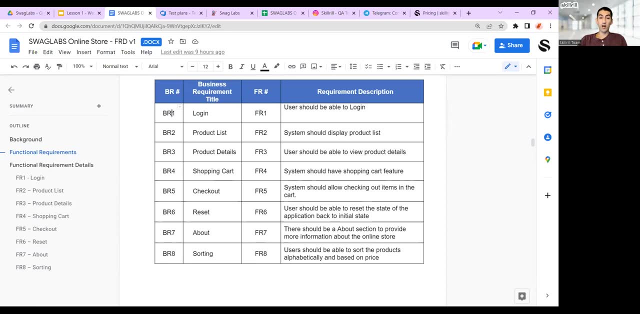 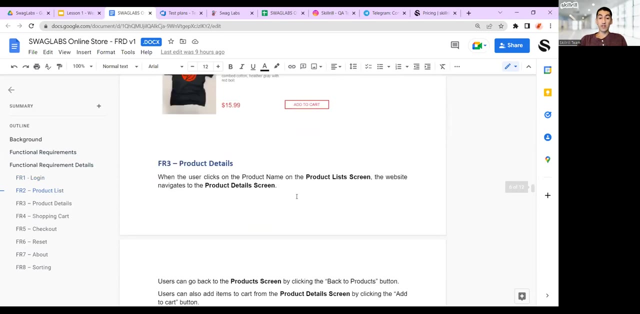 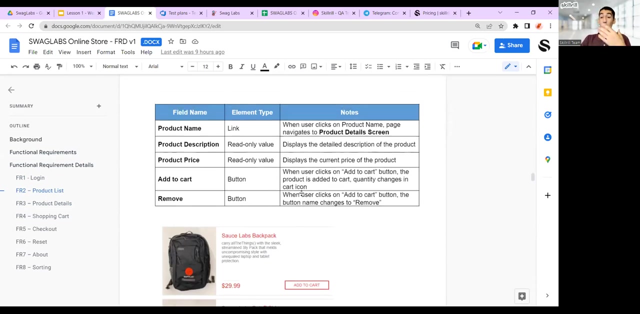 So scroll down version history. table of contents. There is some you know list of requirements here. There's this traceability between the business requirements, functional requirements, And then you go into the detailed information about each requirement. Now, as part of our teaching courses, we provide access to those documents to our students so that they can work. 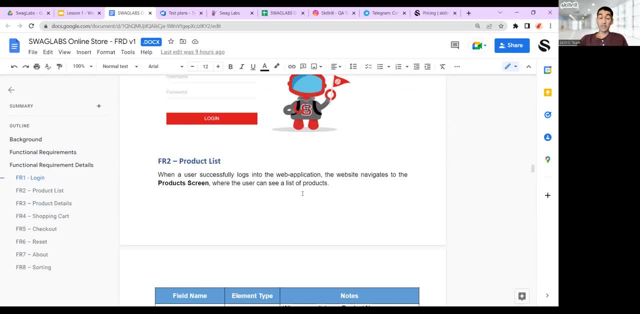 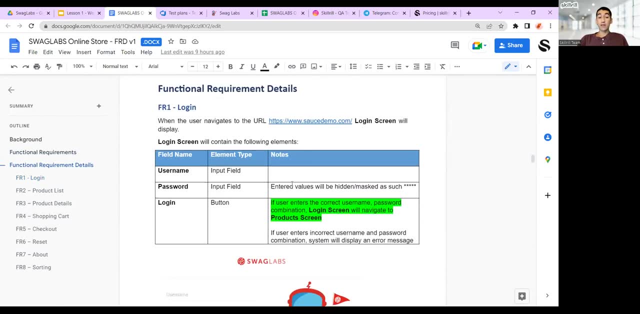 Like In a real work environment, basically so that they can, you know, gain experience, experience, basically. So let's pick the requirement number one, which is login, and start reading. So, as you can see, it says: when the user navigates to this URL, URL means the web address here, and a login screen will display. 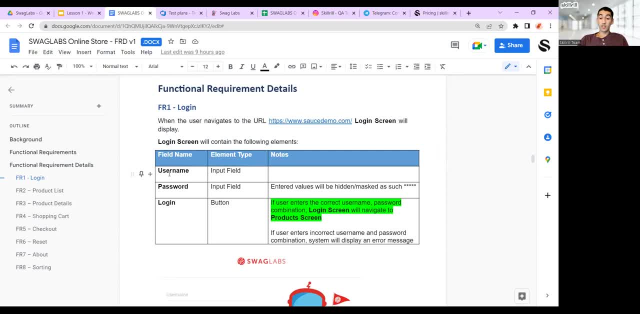 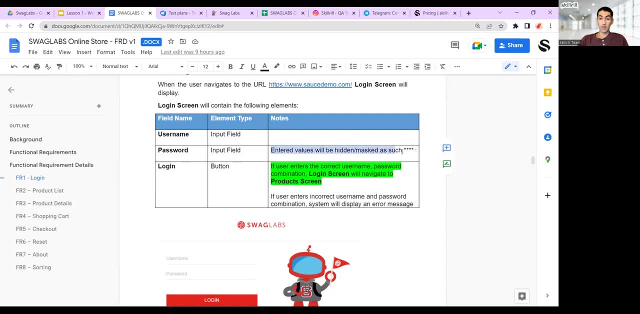 Okay, further, And the login screen will contain the following elements: So we're looking at the username password and the password. Here's one interesting thing you want to pay attention to. Entered values will be hidden or masked as those spells. 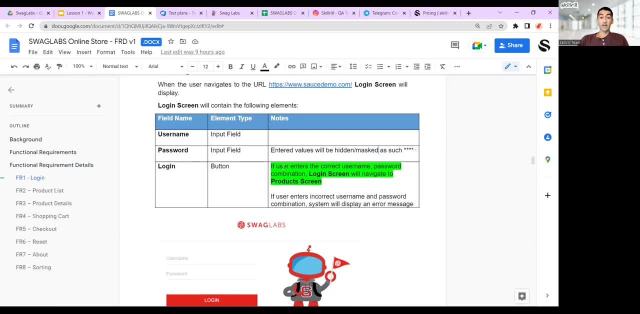 So whenever you're entering your password, it should be hidden Now. login Now. this is where you know it gets interesting, right? So login button If the user enters the correct username and password combination login screen. 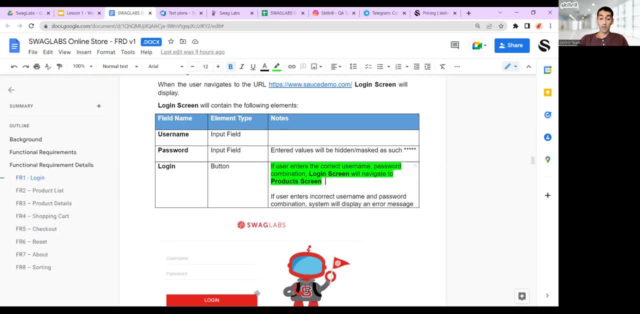 We'll navigate to product screen. This is what we call as a happy path, Sort of right. So correct username, correct password And expect the result. So let's jump into the tool and then create a test case. So this is the main sort of task that you will be doing on a daily basis. 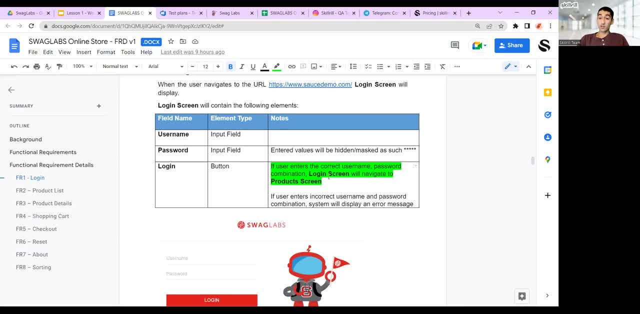 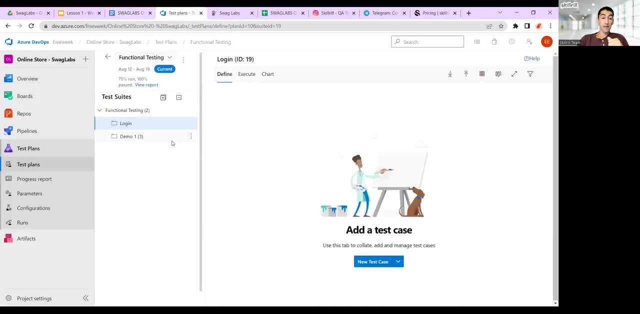 You will be reading the requirements, regardless of where they are, And convert them into test cases, right? So that's what we're going to do. So this is the one of the tools, right? There are different tools in the market. 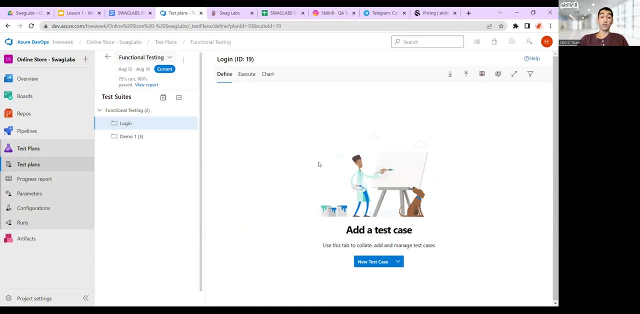 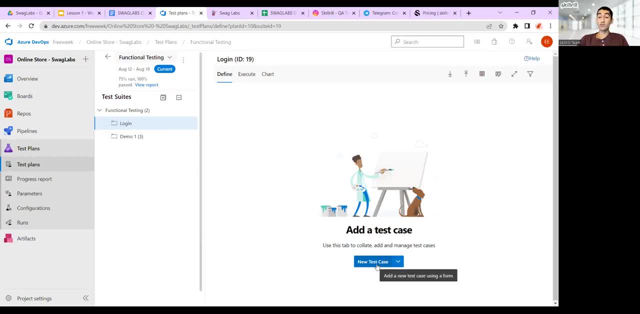 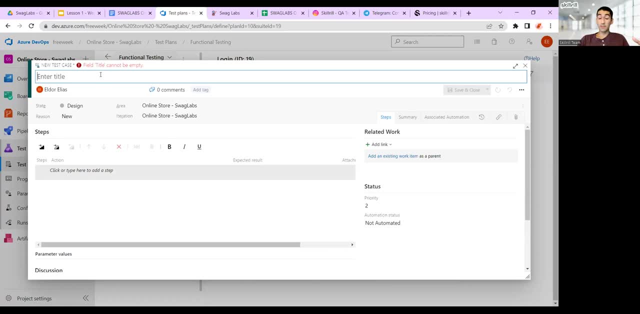 So you're going to. You have this button that's asking you to click on it, So create new test case. So we're just going to go ahead and create new test case And this pop-up window opens. So your first step would be to give a name to your test case, right? 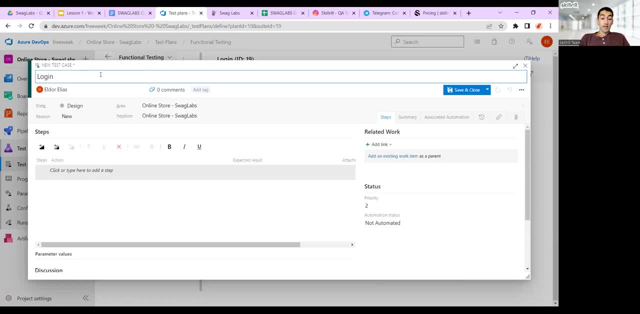 Give a name. So we're just going to name it as login with correct username and password. So some people like to put verify in front of it, Check Test, And I try to keep it clean And I follow the pattern called action plus object. 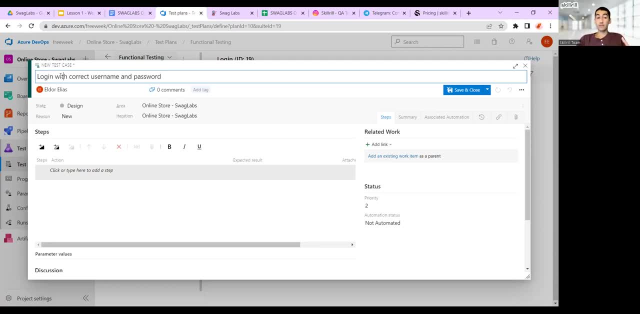 So you just start with the action, like login, And then log into what or with what. So you just mentioned login with correct username and password, And there are other parameters that you can work with here, But we're just going to jump into the steps or actions right away, right? 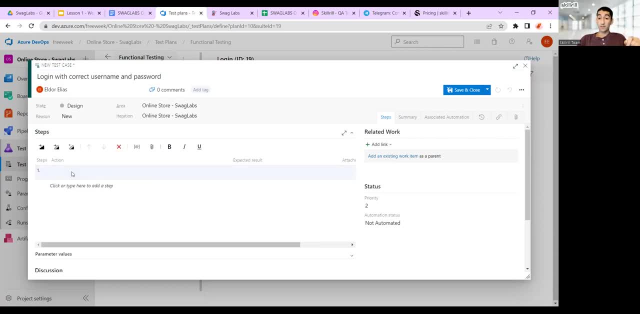 To keep it short, So first step. So what would be the first step? First step would be: we have to open the website, right, We have to go there- And I'm getting some here- Go to the website, Exactly. 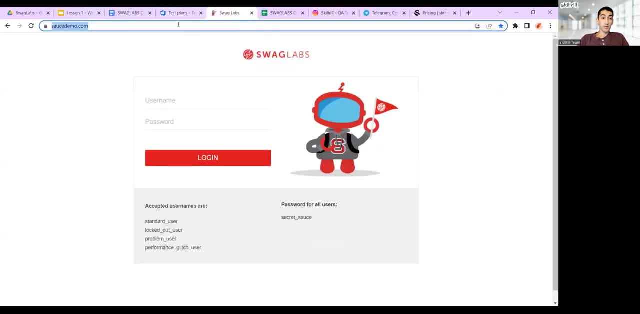 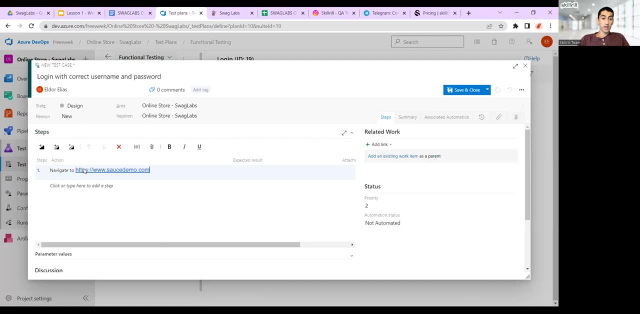 So navigate to. let me just go ahead and copy paste. Actually, you know what This is. we should be copying and pasting from the documentation, That's right. So we're going to copy and paste from here, And the actual result is also described here. 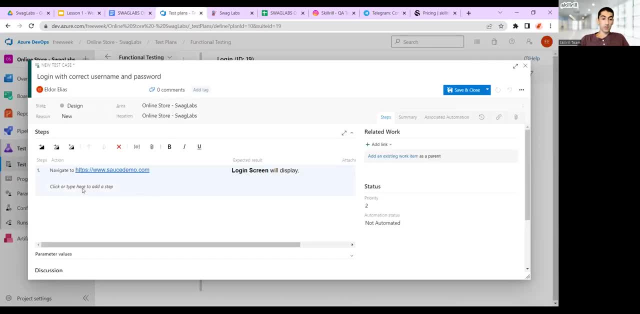 Login screen will display. Let's just go ahead. I'm going to put the actual result. Step two: Enter username, but let's say correct username. right: Enter correct username. What are we expecting? We go here. There's no much expectation here. 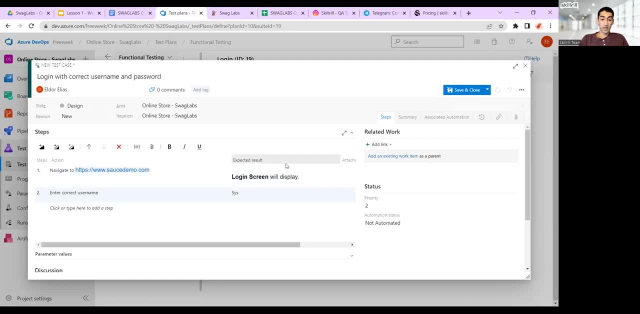 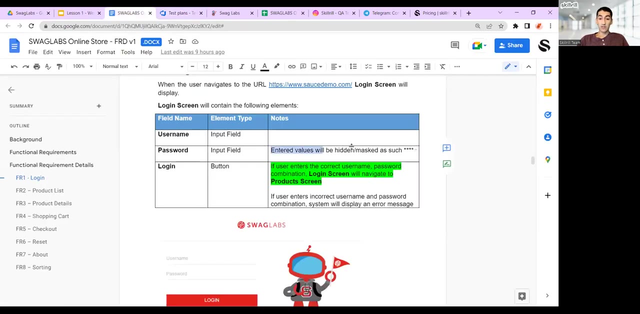 This as long as the system allows you to enter right. System allows to enter Now. enter password right, Correct. Enter correct password. What's expectation here? Let's look at the document. Entered values should be hidden or masked. 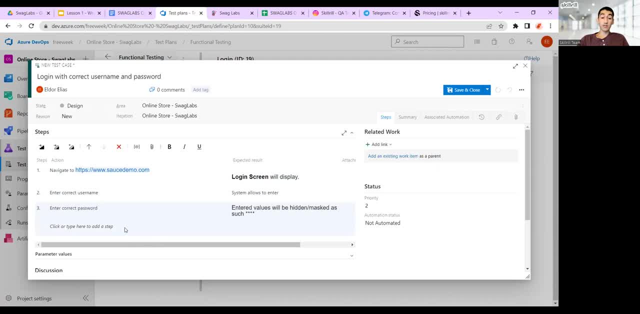 Okay, That's our expected result, or expected result, That's right, Right, So let's go to the step four. That's which is the most, I think, critical part. Just click on login button. So what's expected condition here? 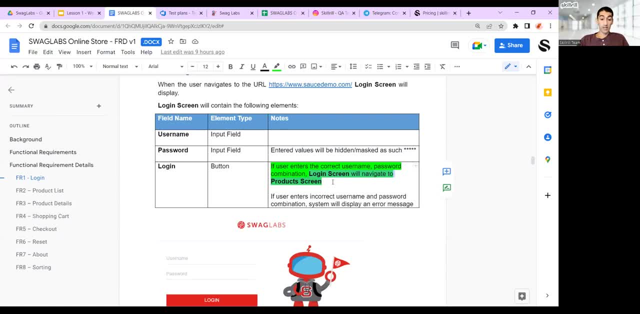 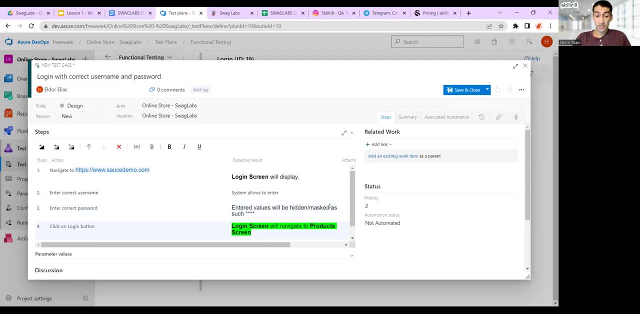 I mean the expected result here, which would be login Screen will navigate to product screen. Let's put that. That's it. So your test case is basically complete, right? So we just took the requirement and then converted that requirement into a test case. 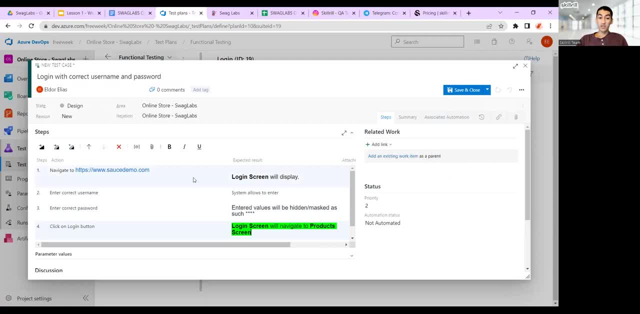 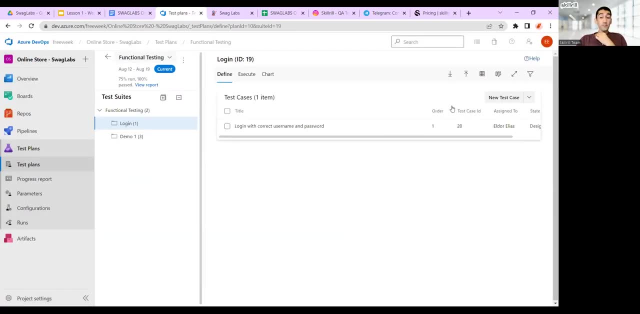 So we have the test case name and we have the actions and we have the expected results. Looks simple. Let's save and close. Now your next step would be- I mean, normally, you would actually, you know, create all your test cases and then execute. 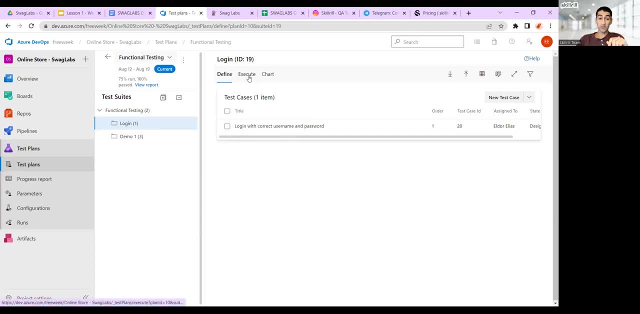 But for demo purposes, I'm just going to go ahead and run the test case for you as well. So we're going to go here and then select, So you're going to go to execute. You see, you can define and then you can execute. 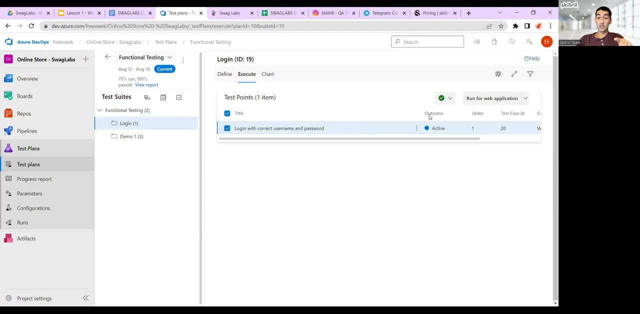 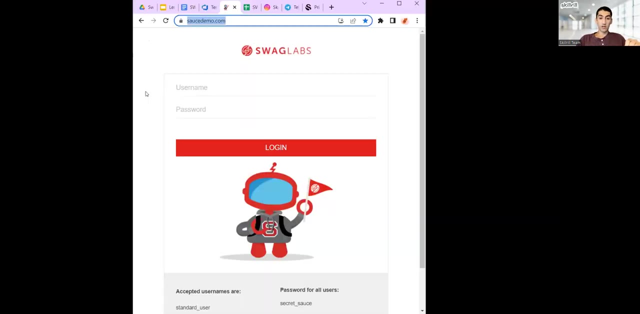 We're going to go to the next tab, execute, and then click run for web application And on the left-hand side here, if you can see this pop-up window open and we're going to open the actual application also on the right-hand side here, right, 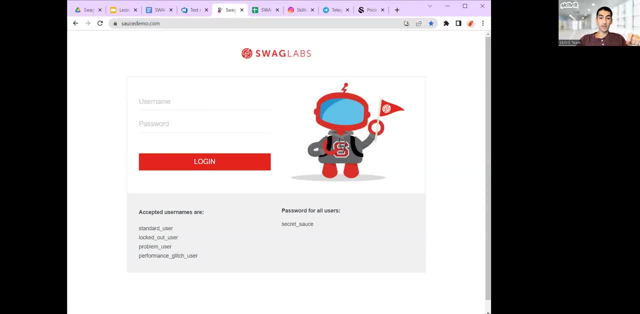 I hope you guys all can see, And then we'll start executing, right? Okay, great, You can see, So we'll start executing. So the first step: we navigated. that's right. We navigated to this website and we got the login screen pass. 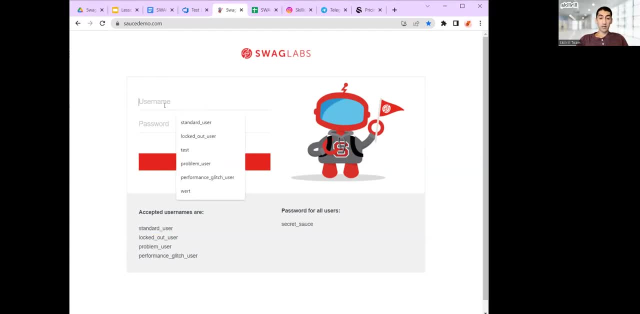 correct username. we're going to get this correct username from here because this is a demo website. all right, it just it allows me to enter. next one is enter the password. let's enter the password. it is masked. it is masked, it is hidden. you know, that's like a, you know industry standard. 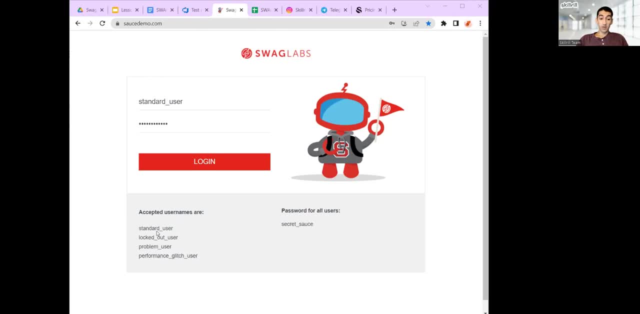 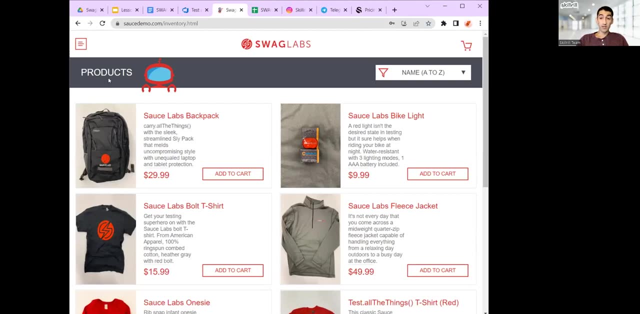 then click on the login. all right, so the next step would be: we're going to click on the login and it took me to the product screen. i didn't see any error message or anything, anything you know out of the ordinary. so you know we passed, so we're just going to pass everything. and there's a button. 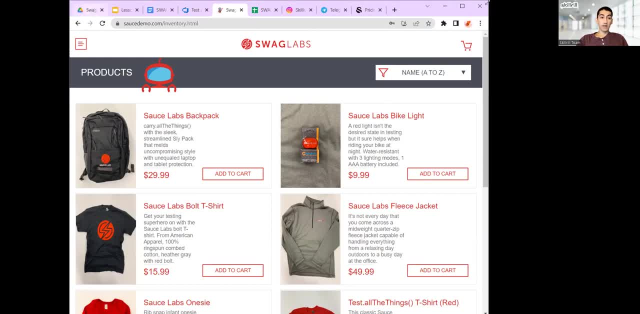 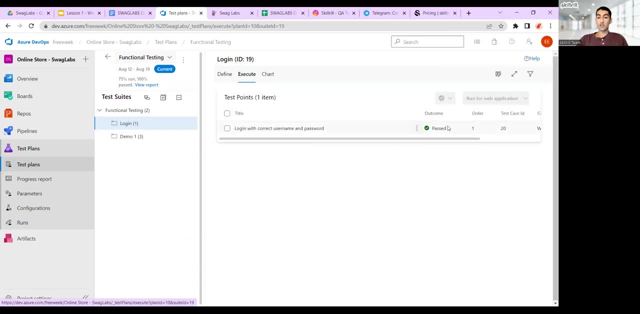 called save and close and we're going to go back. let me enlarge and go back to this here. let's just refresh, go back and you can see the test case status actually now passed. right, so now, um you, so this was your happy path. now let's go back to the documentation and look at the 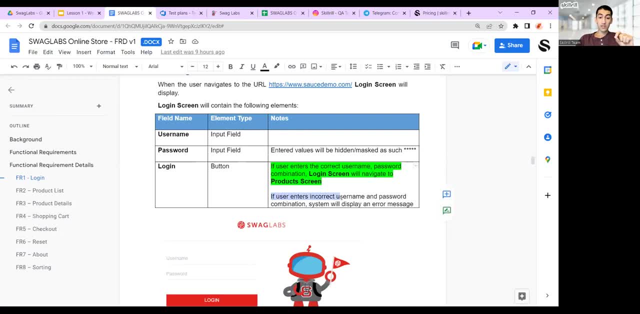 next paragraph here, which says: if user enters incorrect username and password, combination system will display an error message. so so this is more of a negative path, right? if you enter incorrect username and password combination system will display an error message. now here's a question to the audience. 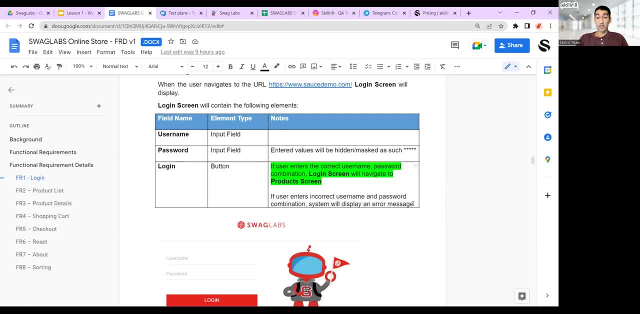 um, what does it mean? incorrect username and password combination, and how many different combinations you could actually come up with? you know, how would you actually test this right, because it's not really telling you. you know, is it one combination, is this two combinations? and how would you test? 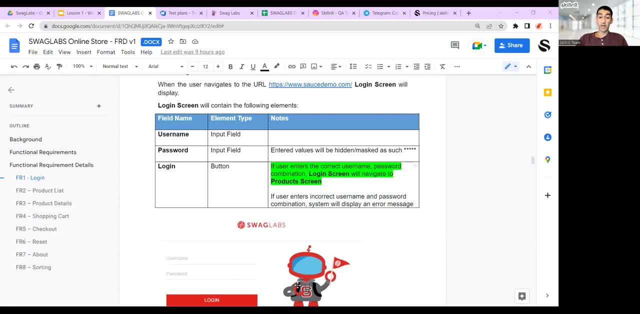 right, correct name and wrong password. here's one, one answer. great, right, correct name and wrong password. you could do that wrong name and correct that. yes, you can. you can flip that, that's it all right. yes, how about a blank username and then you know correct password, or? 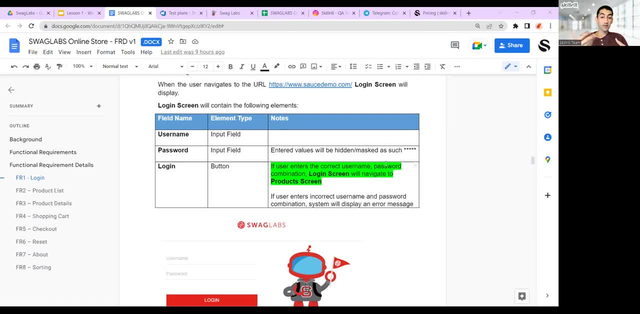 whatever password, right, blank password or populated username. so you see, this is where the tester's knowledge or, uh, professionality, uh, professionality actually, yes, blank- can be considered as incorrect as well. right, so you have to come up with the scenarios. now you have to go beyond the documentation. 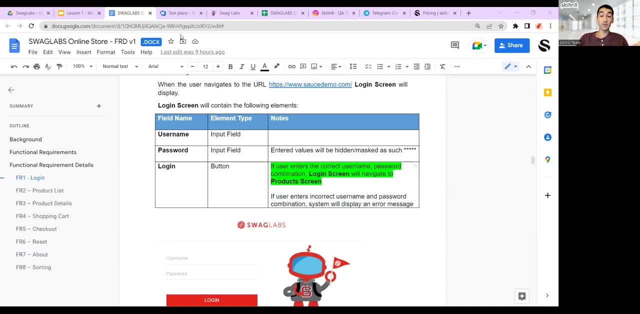 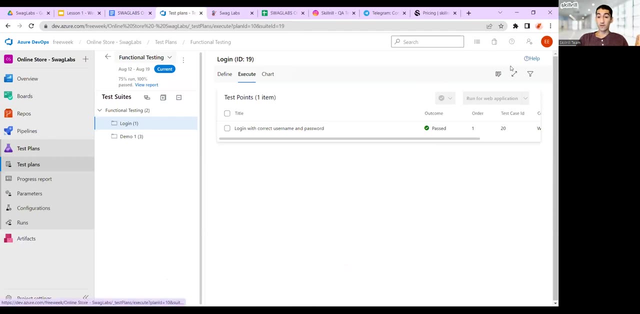 in this particular cases, right, so you have to be able to have, you need to have this break uh to test uh ability. yeah, it may make passwords with numbers and symbols great suggestions. so let's try to create one of those uh additional test cases here. so we're going to go ahead and again click on the 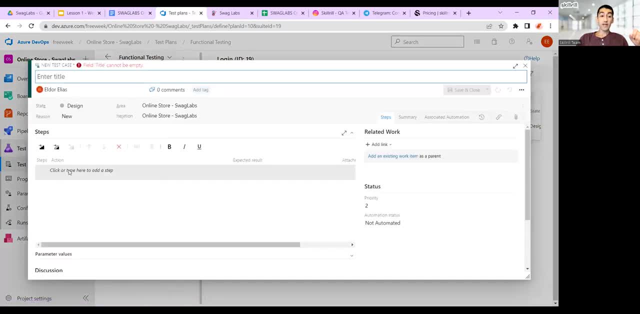 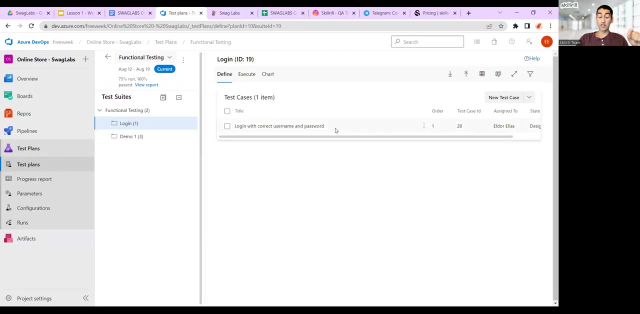 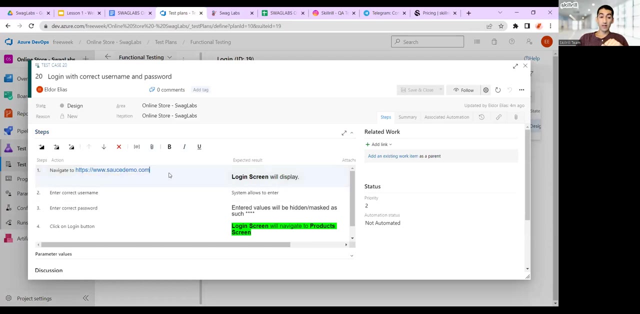 new test case. so, and again same step. but there's one interesting, um interesting, uh concept here that's called shared step. so if you go, if we go to this particular test case that we created here, right um? so let's, let's just go back and then let's create our new test case, right? so here. 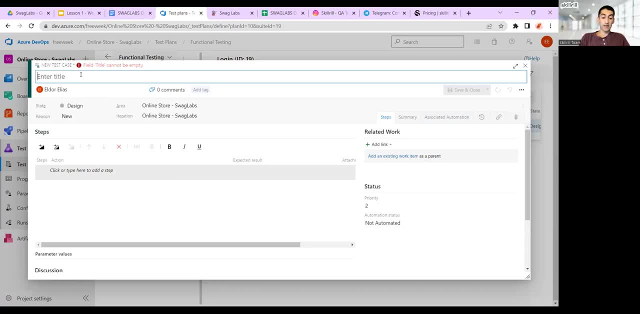 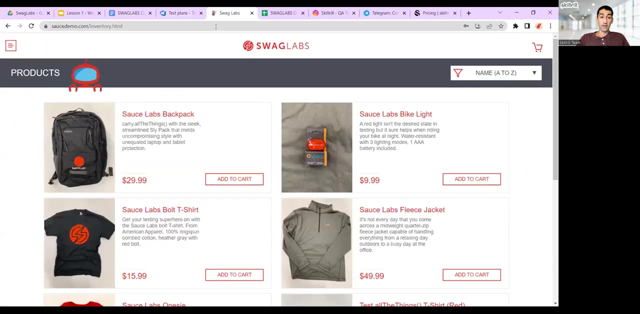 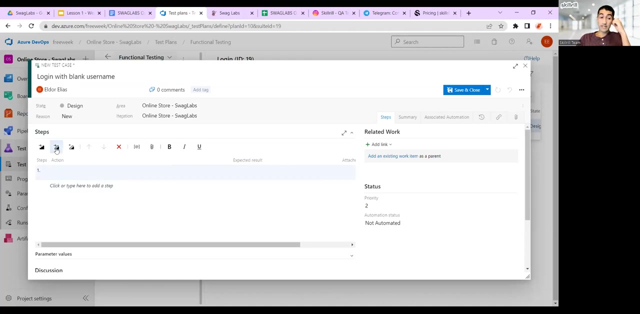 we're gonna uh name this test case as login with blank username, for example. right, this is just one um example of the incorrect or invalid scenario, right? uh? so the first step here again would be navigate to the the website. now, actually, this particular uh step can can be taken, uh, from reusable step, that's. it's a concept called shared step. 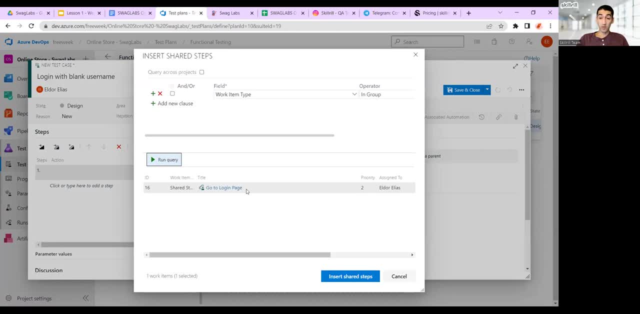 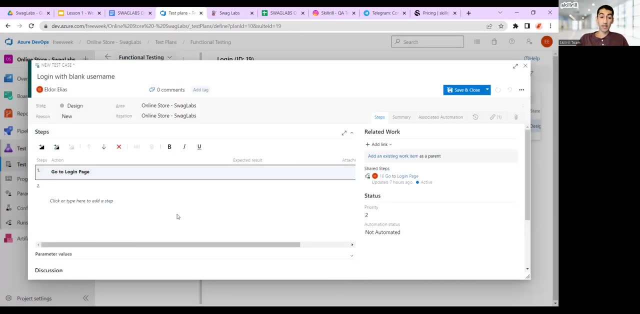 and if, um, you can create shared steps in in most of the test management tools, so that it makes your life easier, so that you don't have to recreate and then redo the same step again and again. as you can see, i just took one of the shared steps, uh, that i created previously and then this gives: 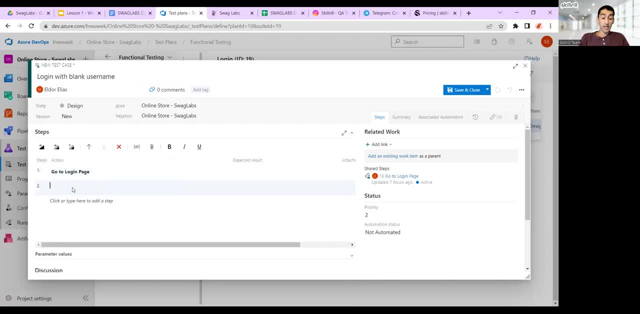 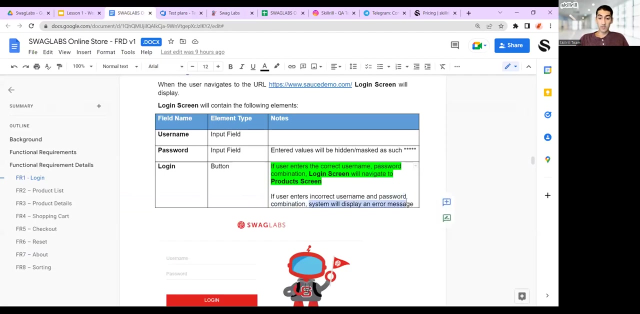 me. this step auto populates the step uh, basically. so the next step here would be: i'm just going to say, leave username as blank and click login button, right. so what's the expected result here? expect result here again: uh, we're going to go back to system should display an error message. now, we don't know what kind of error message. 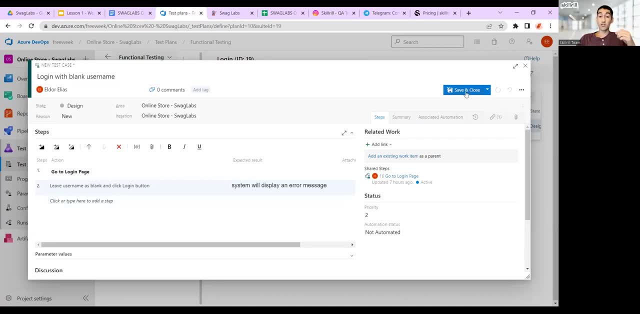 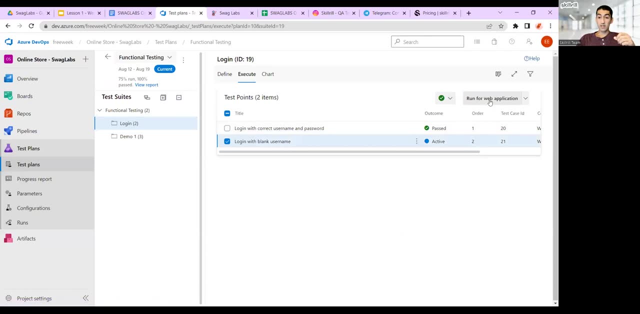 but certainly it should not let you in, right, it should not let you in. so we're going to create our next test case here, and we're going to create our next test case here, and we're going to create our next test case here and run that test case. 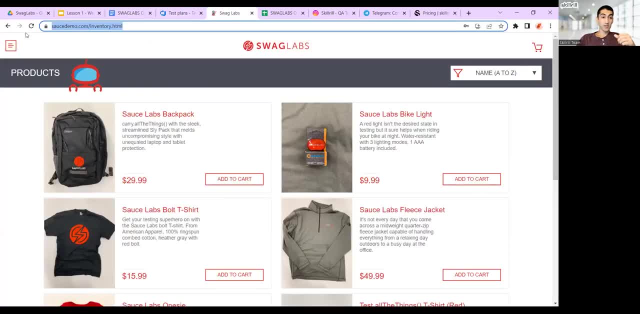 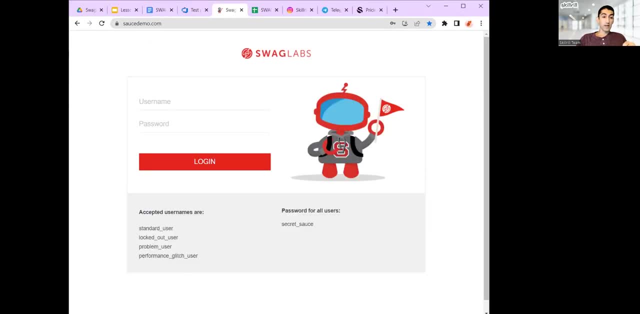 let's log out from the application for a moment. let's put that side by side again. this is pass, right? uh, login is passed, but let's leave this blank. but let's put the correct password here and then click login. you see, you got this. username is required message. 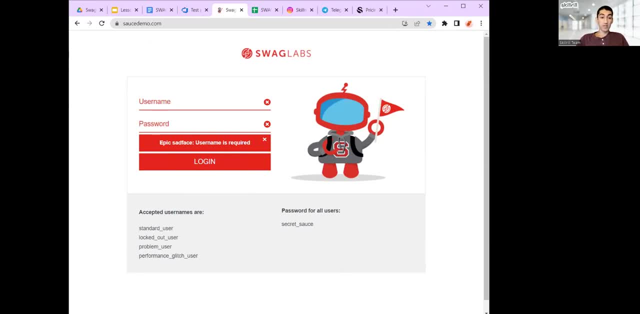 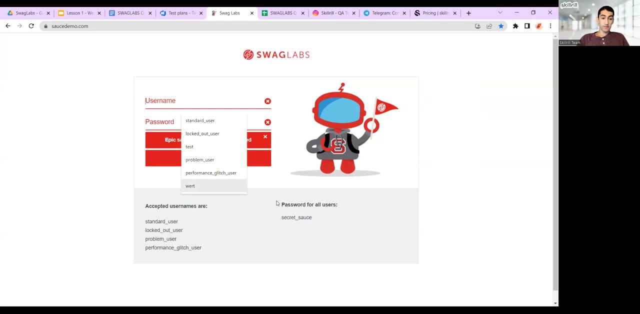 and we could do the other way around, right? i mean, let's just actually complete our test case first. our test case also passed, as expected. now let's explore some of the other options here. and you can leave the password empty as well, right? you click and it says password is required. and what if we just put in two incorrect? 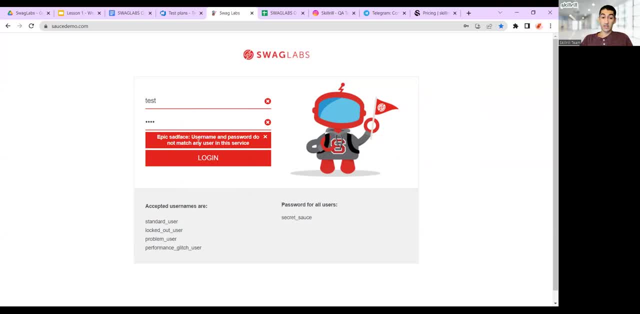 options here and you click on the error message, then you're going to get another error message that says username and password do not match any user in the service. so those are different scenarios, that um, that you could potentially test, um and um, and this is basically how you 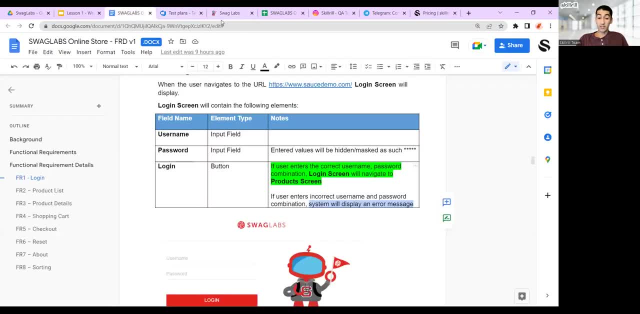 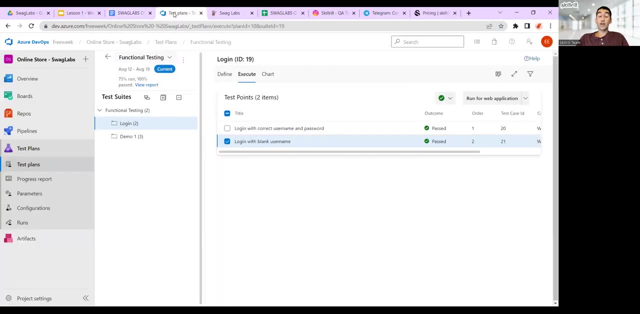 actually going to read the requirement documents and then convert them into test cases- uh, and the- and then run them, and this is one of the tools. uh, certainly, there are many other tools. as part of our teaching courses, We also provide access to the test management tools. so 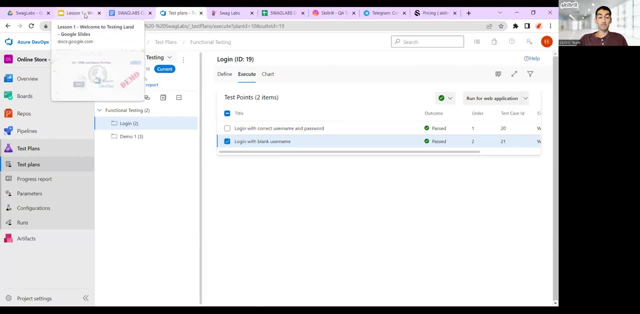 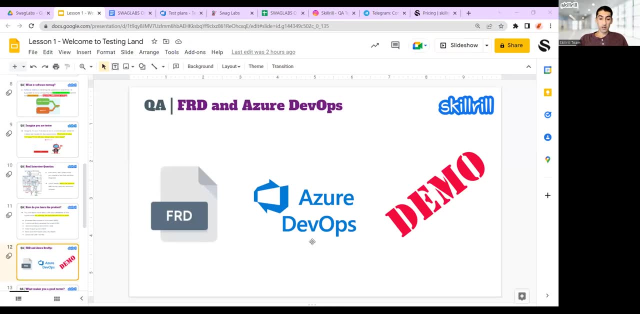 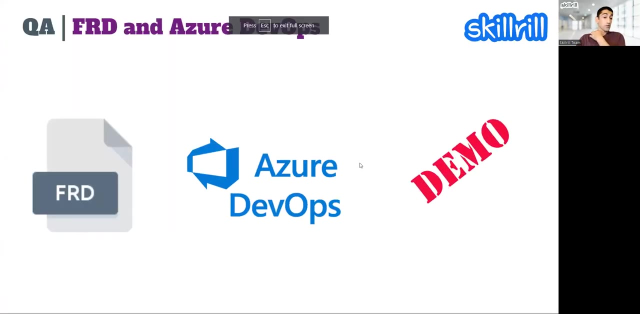 that students can gain experience. All right. So I got some great messages here. Case: no line about password. No line about password, Right, So we just left the. that's right. Yes, I mean, you know you can. you can design your test case in different ways. Certainly you could. 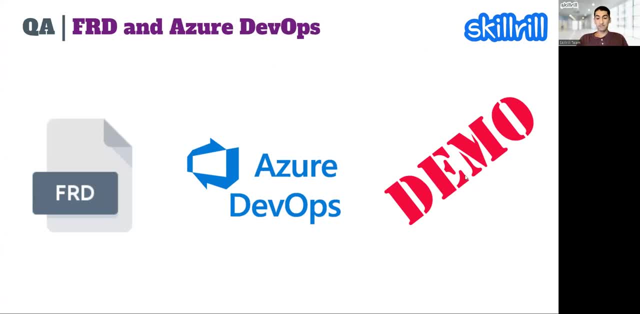 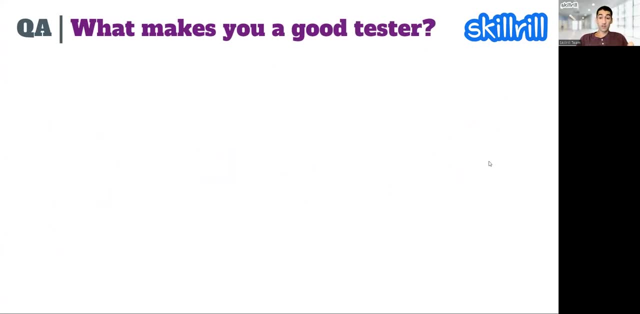 you could split it into different steps and so on. All right, So let's talk about now what makes a good tester right, Before we move on further: what skills actually make a good tester. One of the important skills that a good tester should possess is rapid learning skills. 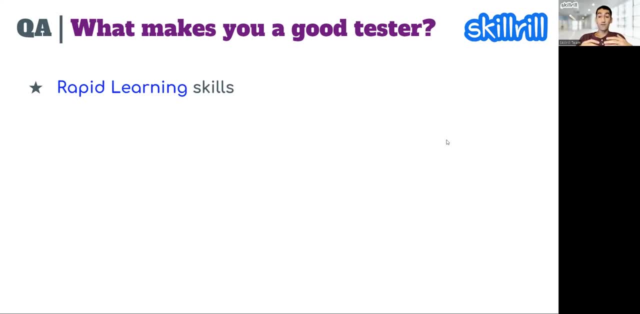 Because you will be given applications frequently, new applications frequently, Sometimes a completely new application that's being, you know, developed from scratch, Sometimes an existing application that you've never seen before, but a small part of the application is being changed And those are usually called as a change request right. No tester actually works in one company. 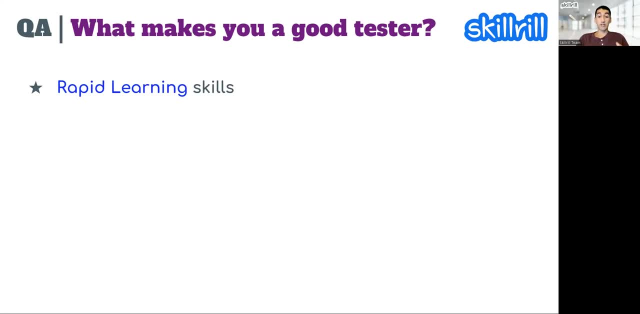 that just works in one project. You're going to end up, you know, working in several projects. You know we hire consultants And then for one year and then we extend them for, you know, two years sometimes, And then. 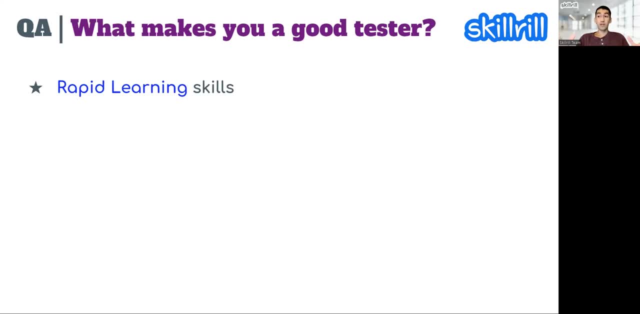 but they end up working during this two years, for maybe you know five to 10 different projects, No, and different, you know, with different testing types, basically, So any. each time you're given a new project, you have to have this ability to quickly learn the application. 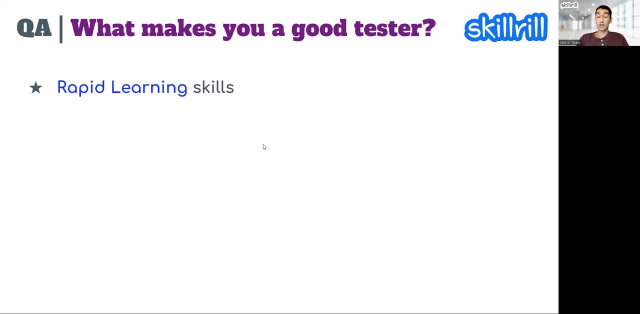 And that's very important- And certainly you know, don't? you don't have to, don't worry if you don't have that skill at the moment, because that's something that you're going to develop over time- that you will be able to quickly look for the correct material. 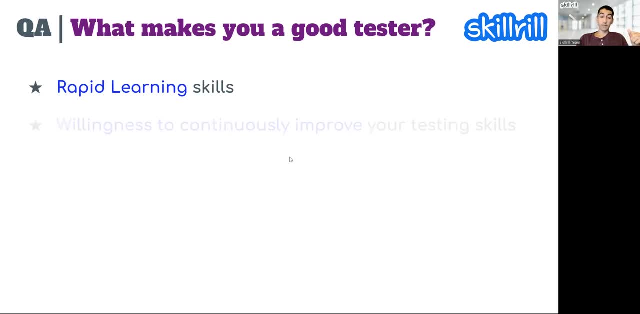 ask correct questions and then understand the application quickly. And then the next important good skill- and this can be actually- this can actually be your interview question as well. right, This can be your interview question. Like what, what do you? 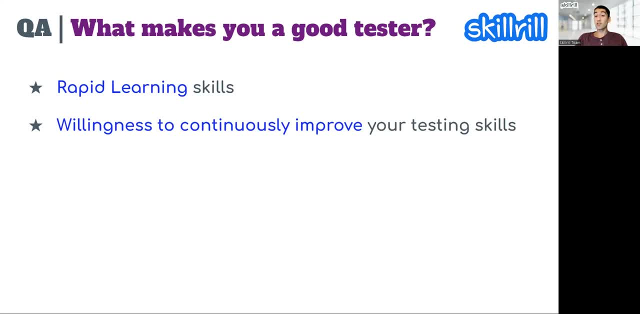 what do you think makes you a good tester? Right, So you can list up. or why do you think we should? we should hire you So you could actually list up those skills as as your own abilities and and behavior. So willingness to continuously improve your testing skills, So you should not. 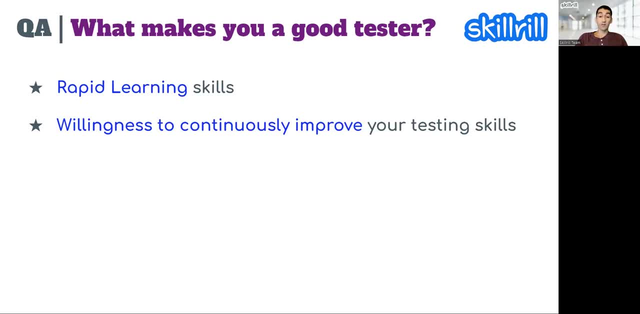 stay in one place and you should always be challenging yourself with new, new tasks and new types of testing and, you know, maybe work on certifications, so that you're always improving your testing skills, because you are in information technologies fields and and technology change fast, right? So the next one. 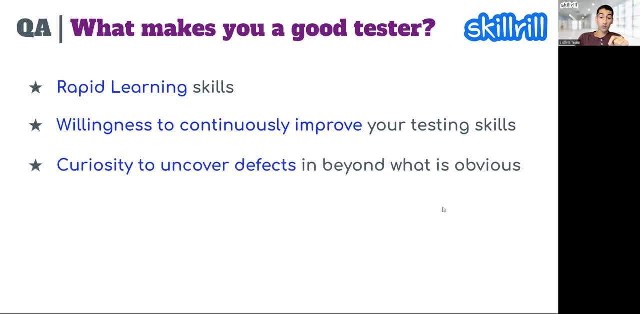 curiosity to uncover defects beyond what's obvious. Curiosity to uncover beyond. why do I say beyond what's obvious? Because the requirement documents or the user stories, you know if you're working in another term or in, in, you know. you know if you're working in an. 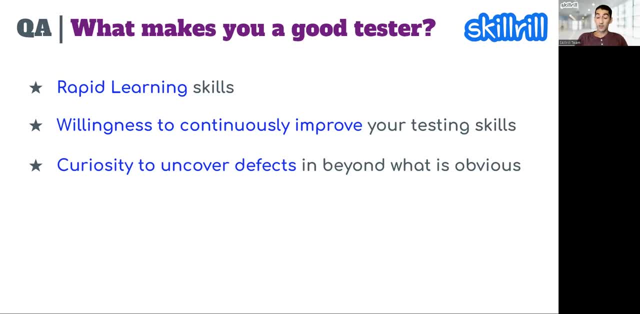 agile environment. those are not always the whole story, right. So there are certain things that are missing, There are certain things that were not actually described as it is, And as a tester, you need to be able to go beyond. I mean, certainly you can survive by just, you know, converting. 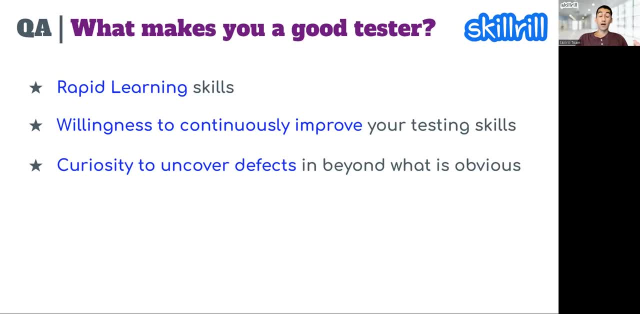 what's written in the requirement document and not going any step further. But I would say, you know, I would say good tester has to be able to go beyond And that's that's. you know, that's that's a, that's a whole purpose of actually hiring a tester. You know you shouldn't be. 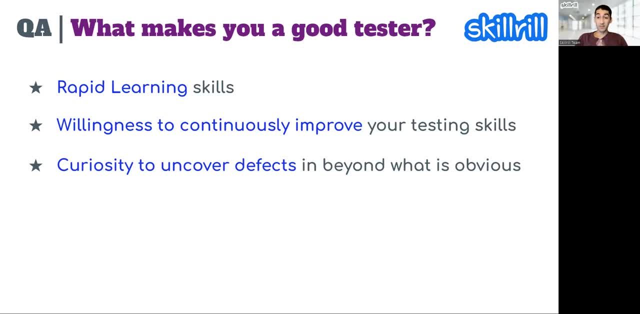 just blindly copying and converting, copying and pasting from the requirement document, like I did actually. So further excellent communication skills. Why, right? Why communication skills are important? That's a big part. It's important because both written and verbally, you will be talking right. Some people say QA testers don't have to talk, or 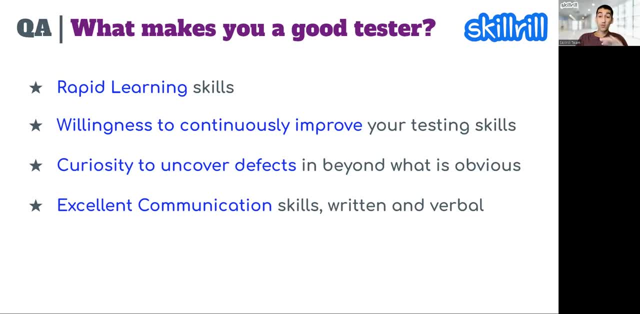 don't have to talk to users and and so on, but you will be talking right, You will be communicating with the developers. You have to explain your thinking process. You have to. sometimes developers call the testers and then ask them to actually explain the defect. 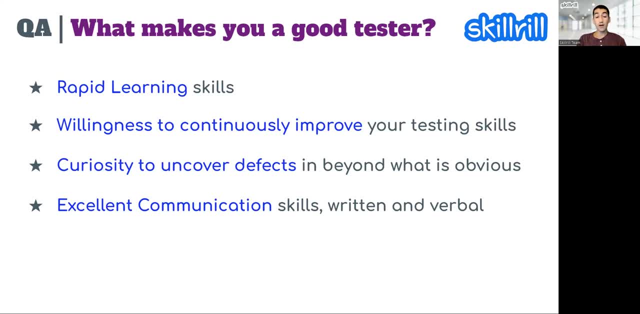 right, We're going to talk about that tomorrow. certainly Any written. you also have to write your defect reports in such a way that it it gets resolved, that it doesn't come back to you saying I'm not sure what what you meant there, you know So. 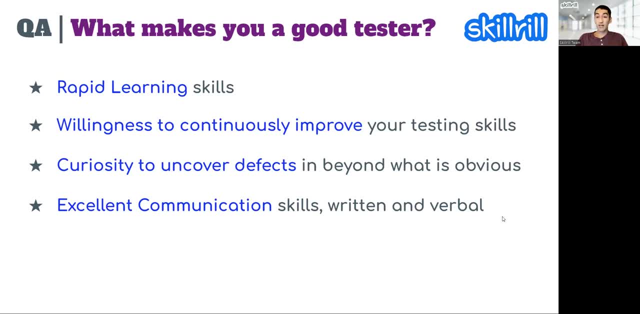 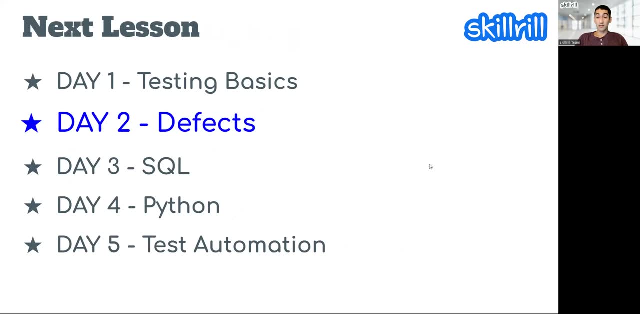 communication skills are very important. You will be talking to the project manager, business analyst and the whole team. basically, Next lesson: defects. right, We talked about testing basics today, So defects is a big one. That's a big part of the QA testing. 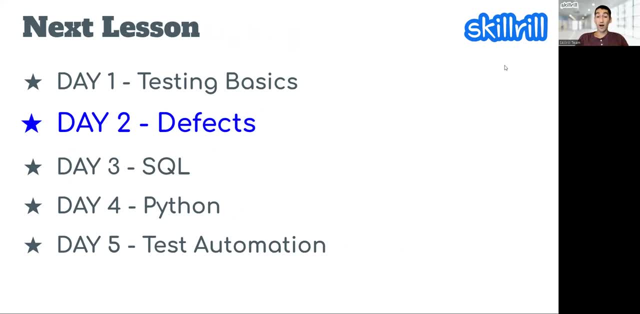 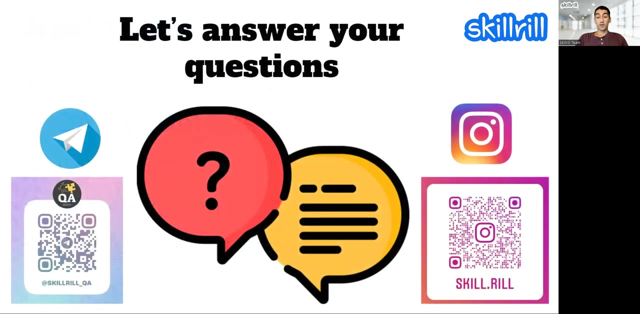 Industry, And this is one of the reasons why this role actually exists, because of those defects, defects that are found and not found. So I would say, you know, stay tuned, and tomorrow, same time, you know, we'll expect you and we'll be happy to share some knowledge. So now let's move on. 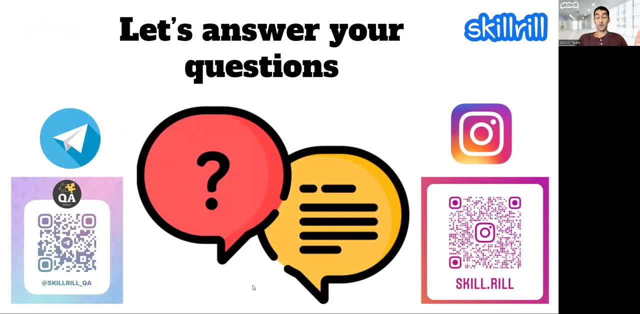 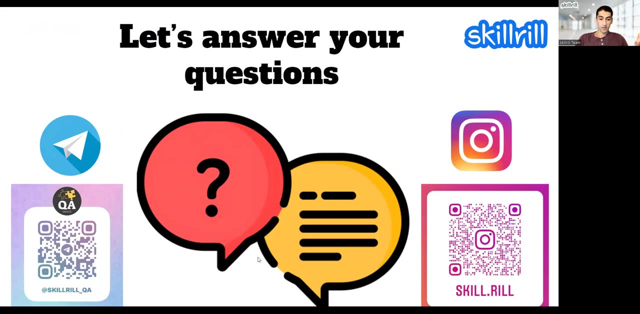 I know we're almost. we hit the time. We have the question and answer session, So let me just go to the questions here. I'm sure it's missed. All right, I sent some questions. Let me just open, Okay, All right. 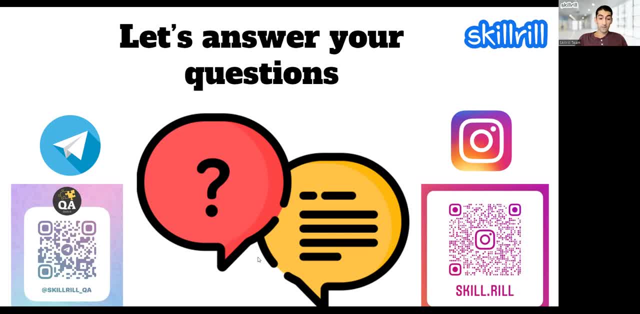 Okay, Yes, Yes, Those are a fast learner. You have to be a good listener. Those are some great comments. by the way, those are the good quantities of the testers. What else we have here, Just see, Can I use Azure dev OPS for API test cases? So as your dev ops? 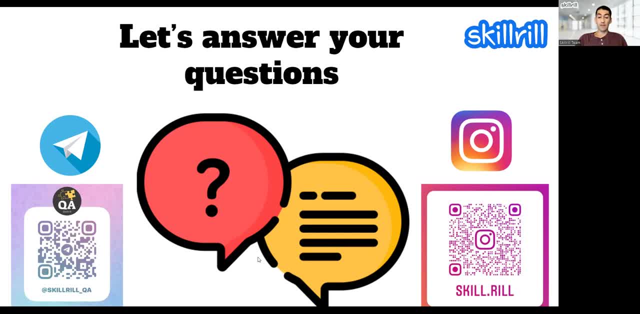 Okay. So, as your dev OPS can can be used for continuous integrations of test software integration in your API. It's not a tool that's specifically designed to perform API testing like a postman, but this is more of a test management tool that has some additional features like. 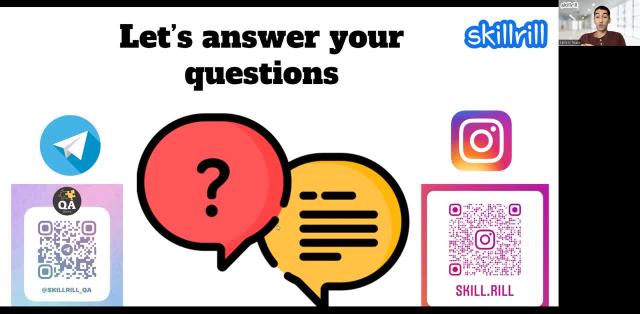 integration with the source control. you know tools like Git and GitHub, And also it has a module called the pipeline And with using the pipeline you can actually create a continuous integration like similar to what you do with Jenkins, I would say. you know Jenkins is. 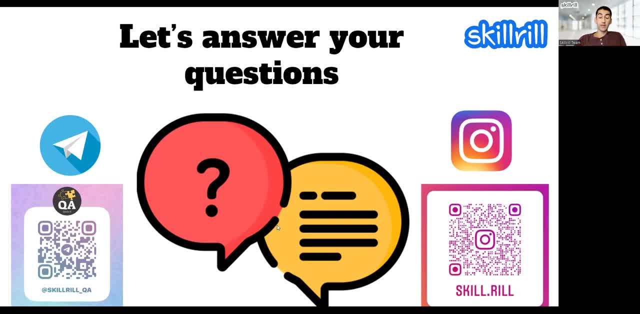 actually, you know it's a lot of headache for the server team. right For the Jenkins you have to maintain a separate server And if you ask me what to choose in between Jenkins and the Azure pipelines, I would go for the pipelines, because that's you know. 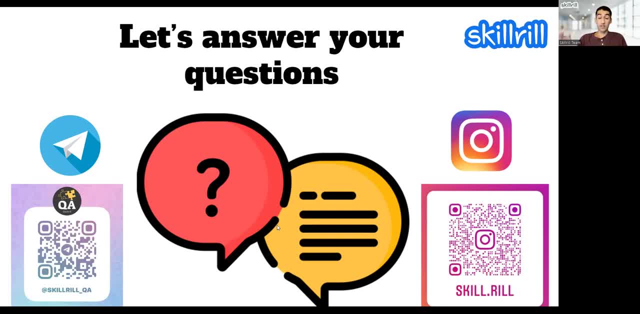 super easy, Super. you know futuristic. basically It's in the cloud, And so that's what we teach as part of our QA course as well. You're going to learn, you know, continuous integration using Python, PyTest and using the Azure DevOps pipelines. All right Questions, All right here, Do you? 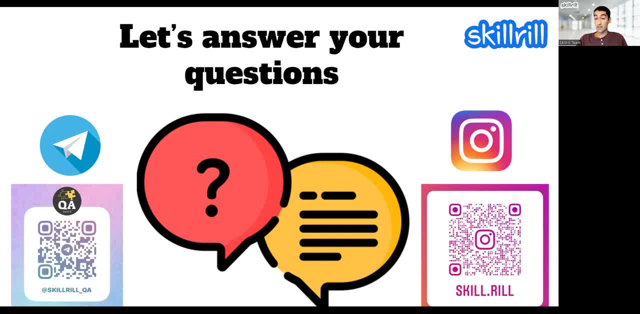 have a course for BA? Great question, Not at the moment. I have some. I know some other bootcamps. I don't know if you have a course for BA. I don't know if you have a course for BA, I can make a referral, you know. just, you know, let you know, just reach out to me, I'll just. 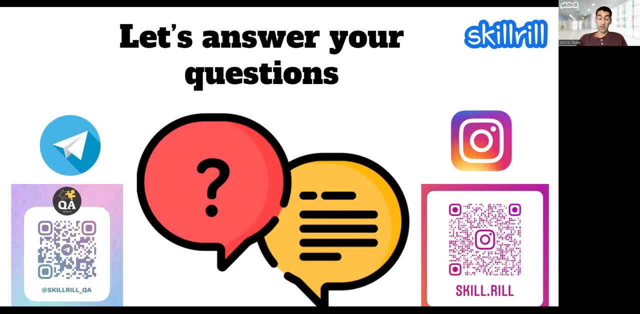 through the Telegram channel that we have, or to the numbers that I shared to the in the presentation, but not at the moment. We don't have BA business analyst classes. All right, And then would the lessons be? yes, lessons would be recorded. These lessons are being recorded. 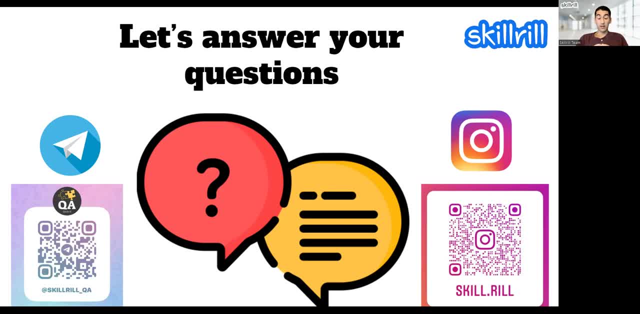 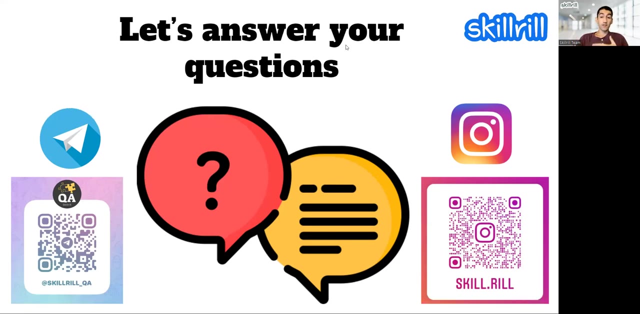 I'll share them with you and the and our future lessons, of course you know. you know the ones that are starting in September also recorded. Okay, Further, how much time we'll be spending? we'll be spending on Selenium, Python and SQL, All right. So you mean during this free session? 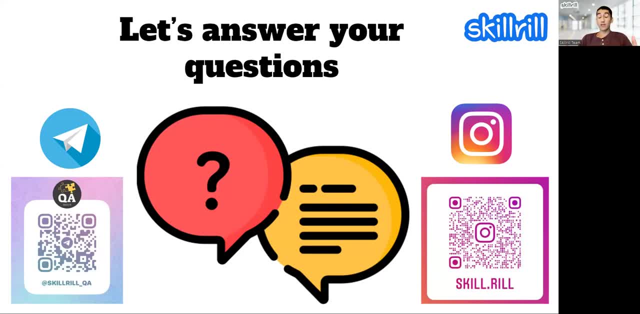 So if we, during these free sessions, we'll try to make them as as useful as possible. So you're going to find out on day. day three will be SQL, And our, our bootcamp is pretty strong in SQL, by the way, because I myself, 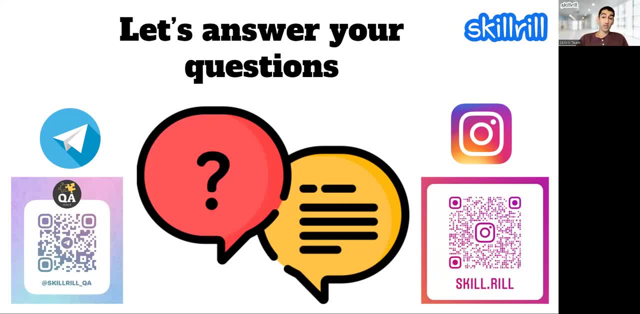 I specialize and there's another teacher who also specializes in data warehouse and ETL and data migration type of testing. So we super strong basically the courses or the, the material is basically super strong in SQL. You know we're, you know I also. that's because also you know the, the way. 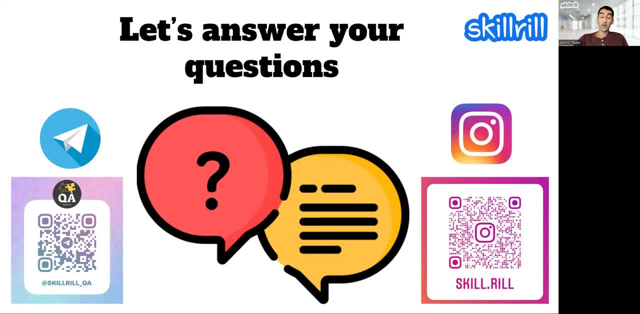 the way I demand from the interview candidates when I interview them as well, cause we have lots of- you know- data with data warehouse related projects And- and I think if you're going as a manual tester, you know your SQL should be strong. 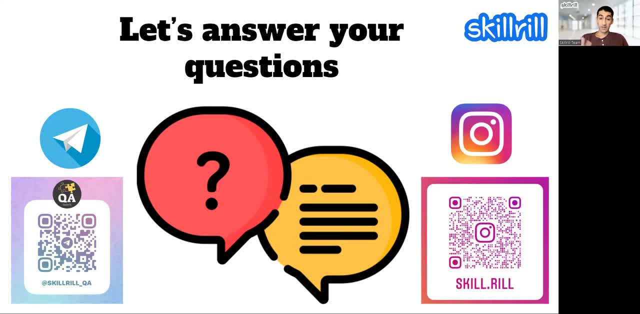 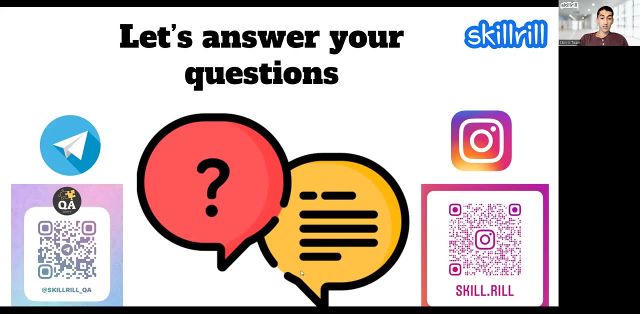 you know, unless you're going for automation, that's that's a different story. but even though automation testers, that's helpful. that's certainly Because these days they're also automating the ETL process as well. All right, So further, I have questions about PostgreSQL. 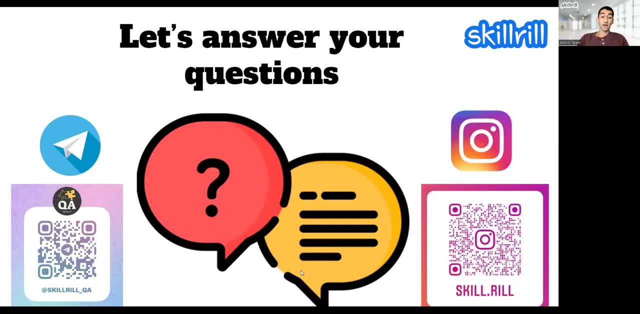 Okay, So there are different flavors of SQL. We mainly teach SQL Server And we're also aware of the Oracle and the differences between them, And some of the resources that we use are based on MySQL. But if you have any questions, you can certainly ask. day three: 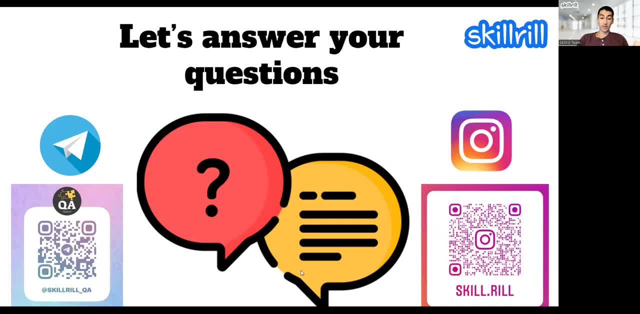 Right. So day three, on Wednesday, you can ask any questions that you have in SQL, All right, So I think I answered these four questions. Let me just go on. Okay, Do you have manual QA? All right, So manual QA course for September 1,. 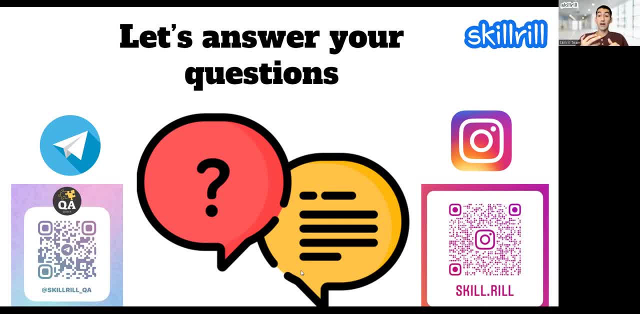 we are actually enrolled. We are currently enrolling for ETL and Automation Manual QA course. we don't have an open enrollment at the moment. For those who are actually thinking of the manual, I suggest to go at least for the ETL plus manual. 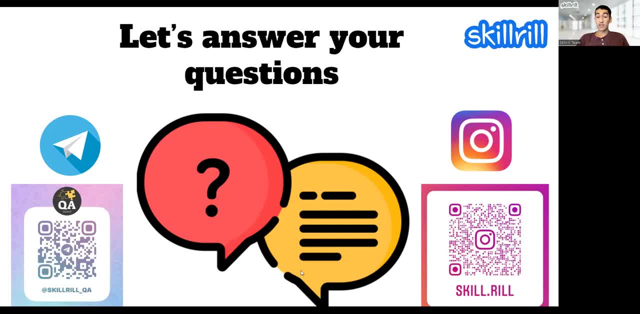 Because if you go to the manual- I mean if you go to the ETL or Automation manual is included, is part of it, Because you can't go to Automation and then just become an Automation tester without knowing the manual testing, because that would be wrong, basically. 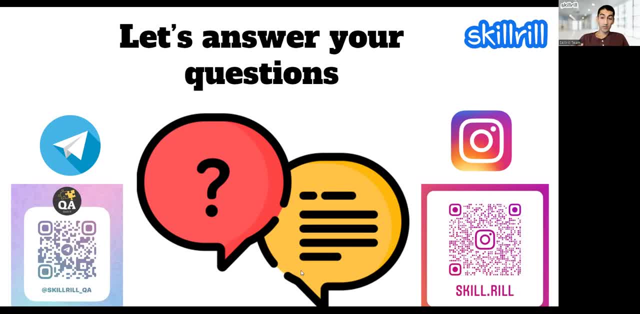 So, and same thing for the ETL testing as well. You know manual testing is part of it. So I would say, go for the you know ETL testing if you really want to go, you know, for manual testing and not for Automation. 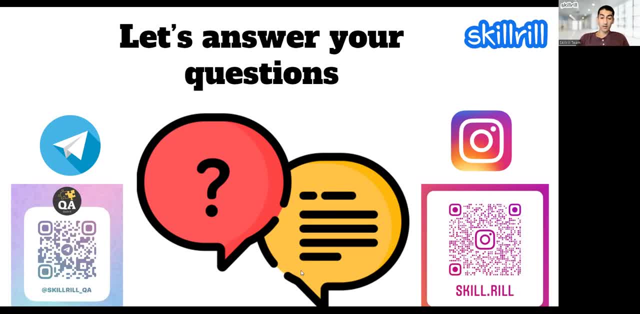 Yeah, sure, Thank you so much as well for your attention here And for your presence here. As far as I know, Python is not needed for a manual. No right for Python is not needed for doing any manual testing, But as part of our ETL testing classes, we provide some 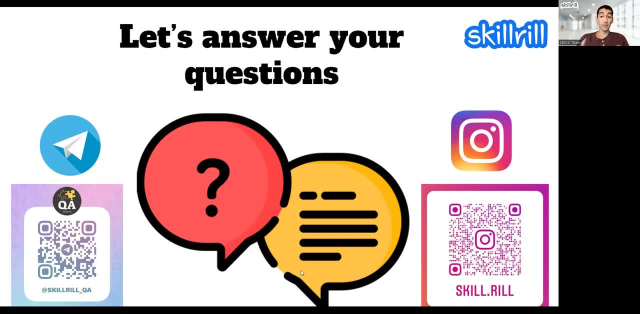 I would say introduction to Python, some basics of Python programming. not test automation, right? Why? Because you know, in the moment, you know, we constantly watch the market and then the industry. What we see, you know, lately, is that the ETL testing positions. 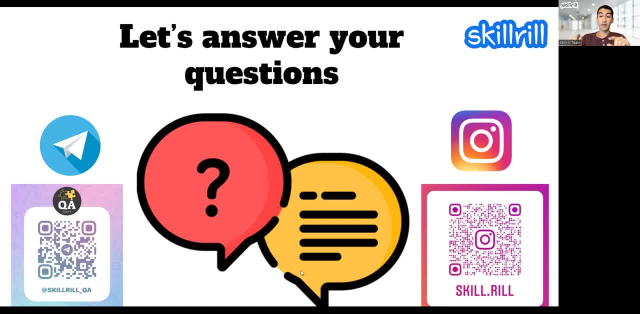 data warehouse testing positions. they are looking for Python skills as well, Because they want to improve that process as well. Yes, you can run SQL queries using Python. Absolutely, You know that's. you know, there's a framework that you're going to create. 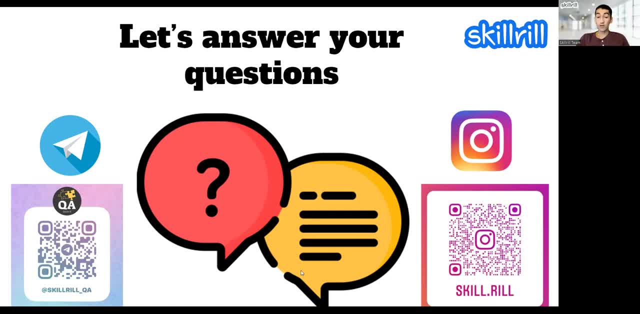 which is called data driven framework, And you can run automatically your SQLs connecting to the SQL server and then you know, report the results, make this integration and all that. So that's the answer to your question, And let me just all right. 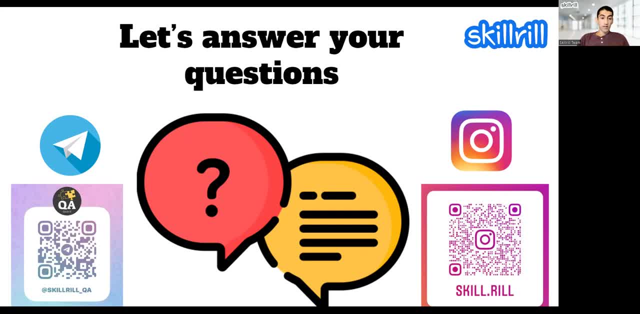 Thanks. Yes, Thank you as well, Jason. All right, So we're going to get to Jason as well? Not certainly. Yes, Jason is part of it. You're going to learn That as well, as as part of your API classes and also as part of your Python classes. 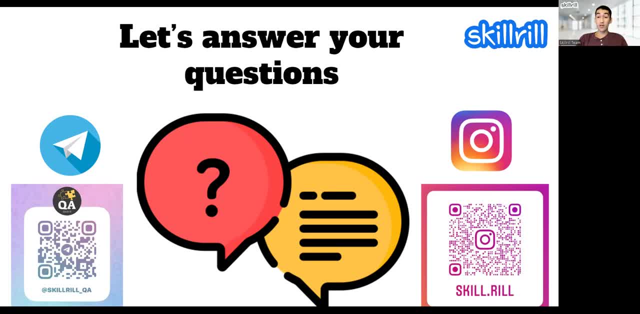 there's a. there's a specific data type called dictionary. That's very similar to, you know, the format of the Jason. actually, Jason is needed. Yes, Okay, How strong SQL and Python knowledge be after the Bootcamp, will it be strong enough for entry level? 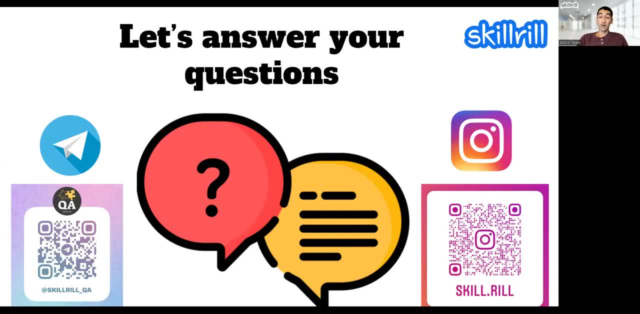 Okay, Yes, it will be strong enough for entry level, I can assure you on that. Yes, So cause you're not just learning saying hello world, you're going to learn all the data types and the object oriented programming concepts and you know, starting from inheritance encapsulation. 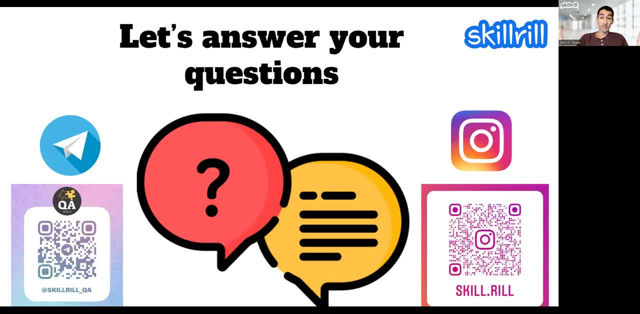 and all of it basically Abstract and all those fancy words, and you will be covered on that part And you will create- independently create- test automation frameworks so that you can talk about explain how you created those test automation frameworks during job interviews. 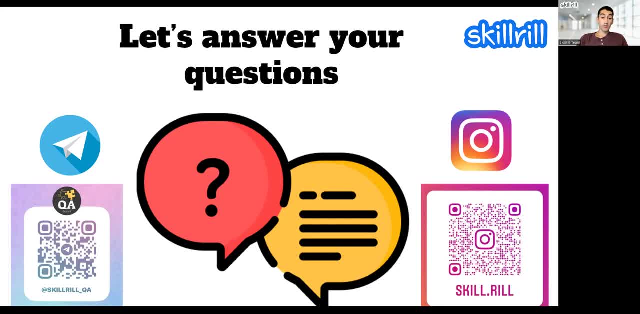 All right, and how much time? how much time we'll be spending on each throughout 300, how much time on each? Okay, so lessons will go in parallel, So we don't teach like you're going to learn SQL a little bit. 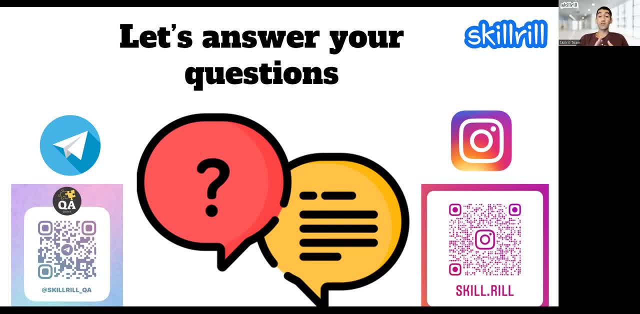 and then just forget about SQL and then focus on something else. So it will actually go in parallel, so that you're always a little bit of everything, but with a full focus on your specialization. So if you're learning, if you're in the automation, 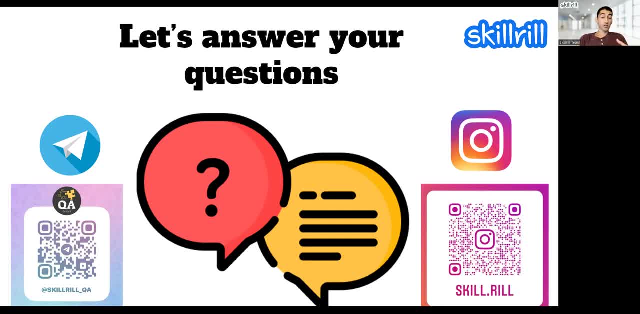 so, right after the manual, you are going to go into automation and you're going to go into automation And that's going to be your core. but along the way we'll give you additional information: SQL and the manual, testing basics and the interview preparation, so that you know you're prepared. 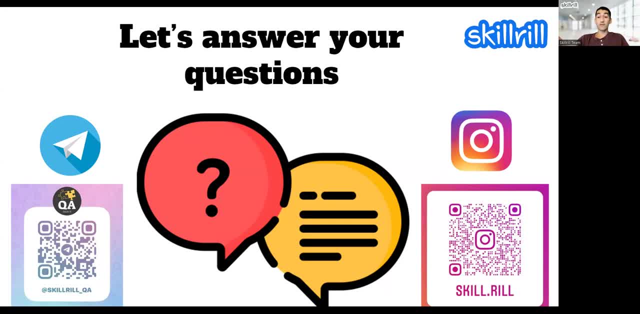 along the way and then you just take everything together, right, If you just learn SQL at the beginning and then just you know, don't come back to it another five months, you're going to forget about it. So Do you get a certificate? 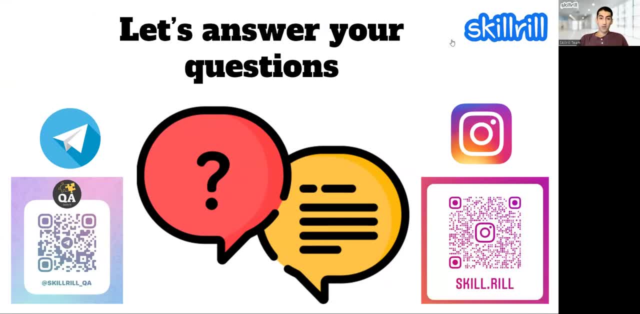 Yes, you do get a certificate. All right, I think I answered all the questions here. And what time are the classes? So, if you're asking about this classes they're going to start in September. Usually starts at 730 or 7 pm. 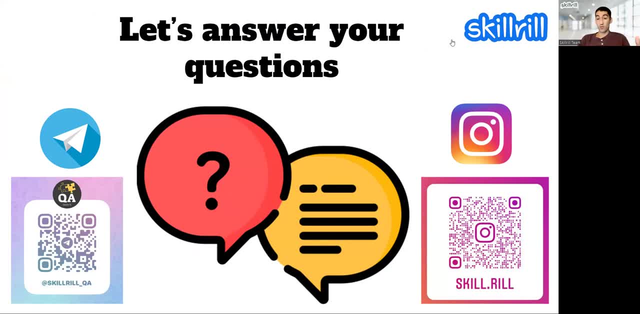 Eastern time. but it depends on the group as well, right, Depending on the group And the majority, The majority of the group, and then where their time zones are, we're going to adjust accordingly And we're certainly going to go, you know, try to meet your needs in that. 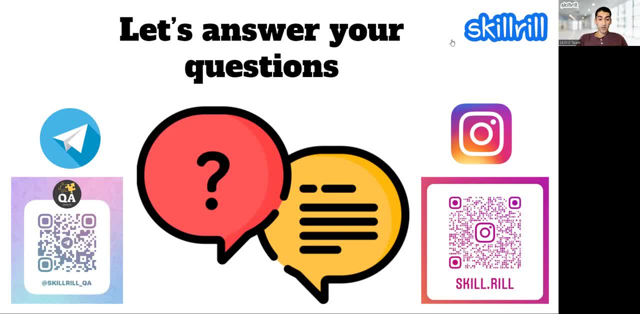 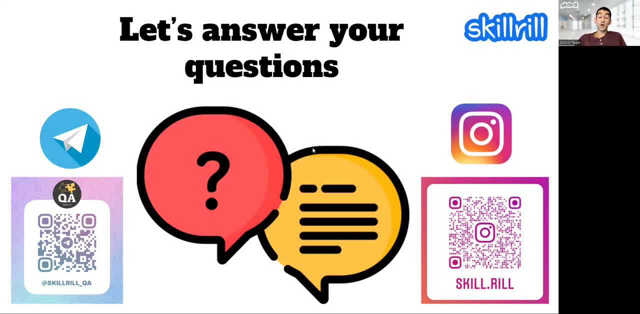 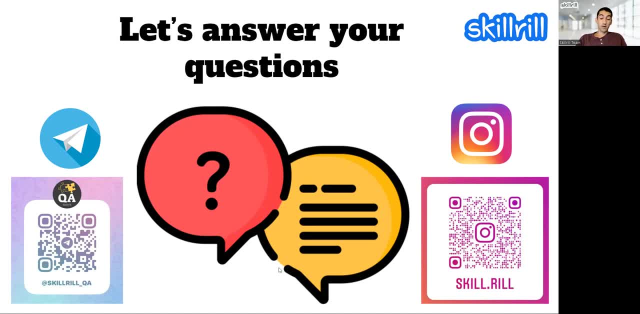 where you can, you can call us, and you also had this uh number in the uh, let me actually uh put the number as well so that you can call. so this is the number that you can reach out to to get more information. um, and you have yet, if you 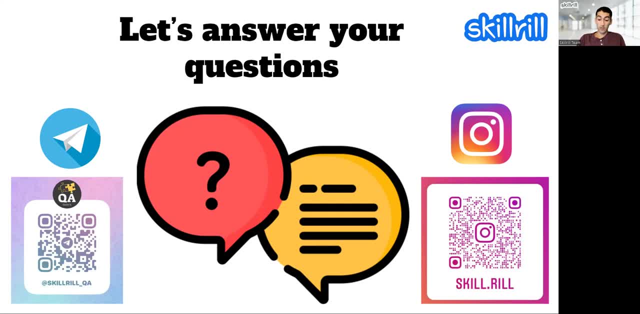 have any additional uh questions? uh, so i can put my own number here as well. so here's the second number is my own number. if you guys have any questions, any doubts or you need any feedback, and, uh, those are the number that you can reach out to us.